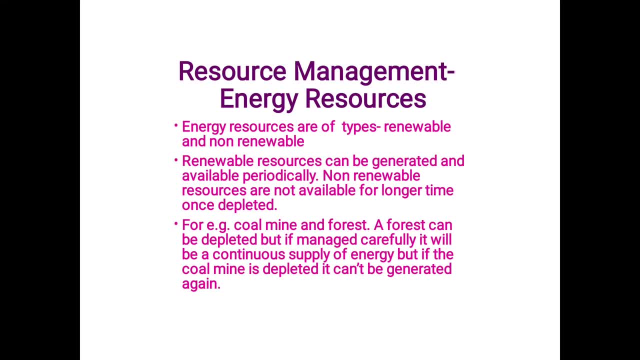 BSC 3, Semester 6.. Name of the paper: Environmental Geology. Name of the topic: Resource Management. Out of that we are going to learn energy resources. BSC 3, Semester 6.. Name of the paper: Environmental Geology. Name of the topic: Resource Management. Out of that we are going to learn energy resources. 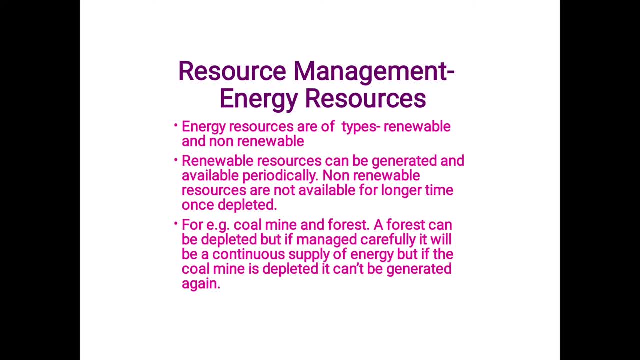 BSC 3, Semester 6.. Name of the paper: Environmental Geology. Name of the topic: Resource Management. Out of that we are going to learn energy resources. BSC 3, Semester 6.. Name of the paper: Environmental Geology. Name of the topic: Resource Management. Out of that we are going to learn energy resources. 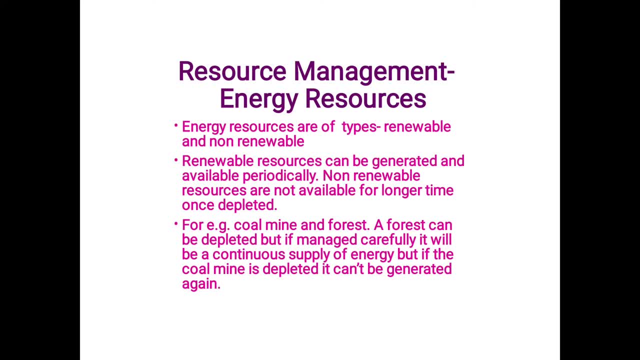 BSC 3, Semester 6.. Name of the paper: Environmental Geology. Name of the topic: Resource Management. Out of that we are going to learn energy resources. BSC 3, Semester 6.. Name of the paper: Environmental Geology. Name of the topic: Resource Management. Out of that we are going to learn energy resources. 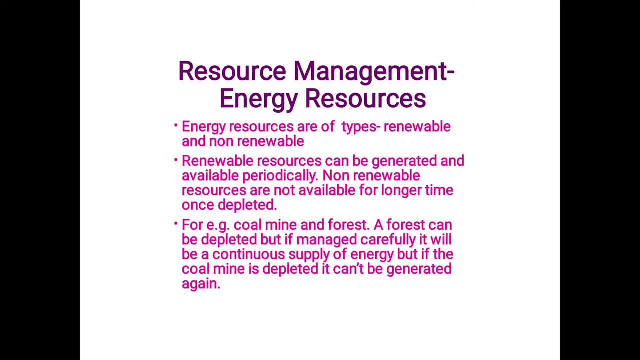 BSC 3, Semester 6.. Name of the paper: Environmental Geology. Name of the topic: Resource Management. Out of that we are going to learn energy resources. BSC 3, Semester 6.. Name of the paper: Environmental Geology. Name of the topic: Resource Management. Out of that we are going to learn energy resources. 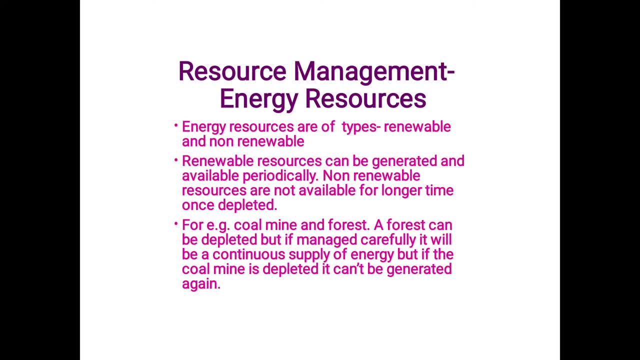 BSC 3, Semester 6.. Name of the paper: Environmental Geology. Name of the topic: Resource Management. Out of that we are going to learn energy resources. BSC 3, Semester 6.. Name of the paper: Environmental Geology. Name of the topic: Resource Management. Out of that we are going to learn energy resources. 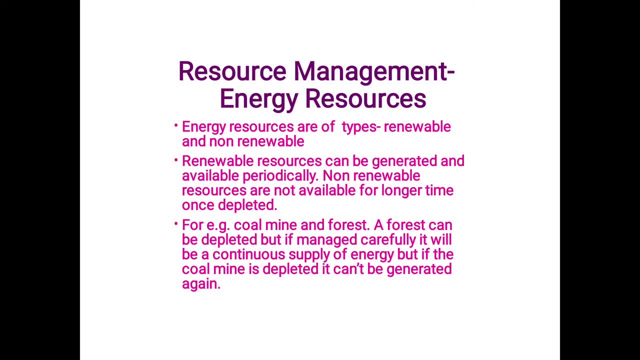 BSC 3, Semester 6.. Name of the paper: Environmental Geology. Name of the topic: Resource Management. Out of that we are going to learn energy resources. BSC 3, Semester 6.. Name of the paper: Environmental Geology. Name of the topic: Resource Management. Out of that we are going to learn energy resources. 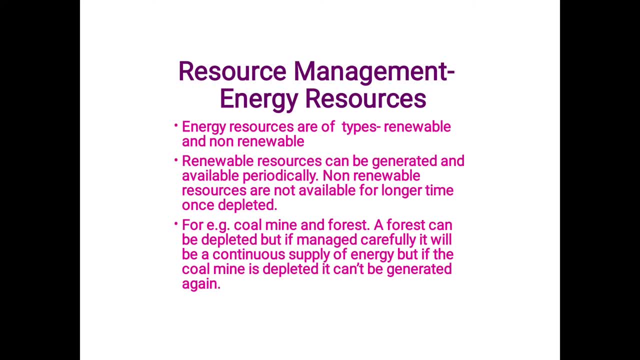 BSC 3, Semester 6.. Name of the paper: Environmental Geology. Name of the topic: Resource Management. Out of that we are going to learn energy resources. BSC 3, Semester 6.. Name of the paper: Environmental Geology. Name of the topic: Resource Management. Out of that we are going to learn energy resources. 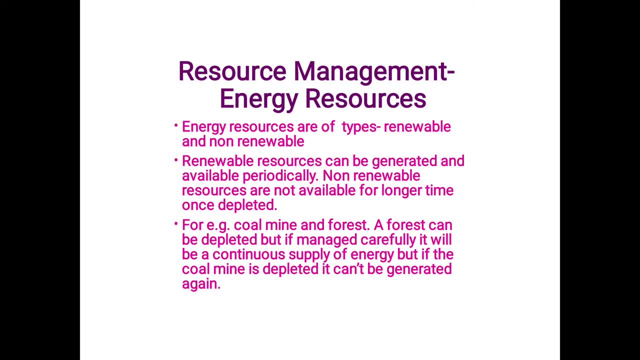 BSC 3, Semester 6.. Name of the paper: Environmental Geology. Name of the topic: Resource Management. Out of that we are going to learn energy resources. BSC 3, Semester 6.. Name of the paper: Environmental Geology. Name of the topic: Resource Management. Out of that we are going to learn energy resources. 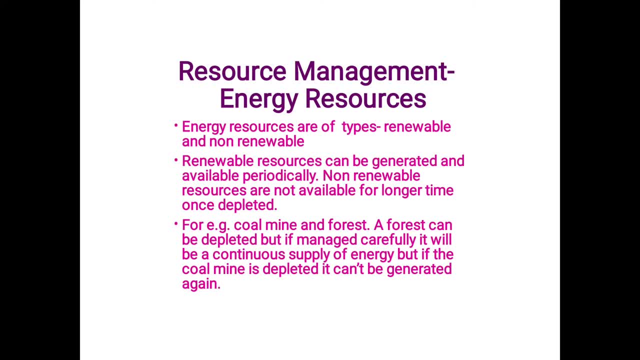 BSC 3, Semester 6.. Name of the paper: Environmental Geology. Name of the topic: Resource Management. Out of that we are going to learn energy resources. BSC 3, Semester 6.. Name of the paper: Environmental Geology. Name of the topic: Resource Management. Out of that we are going to learn energy resources. 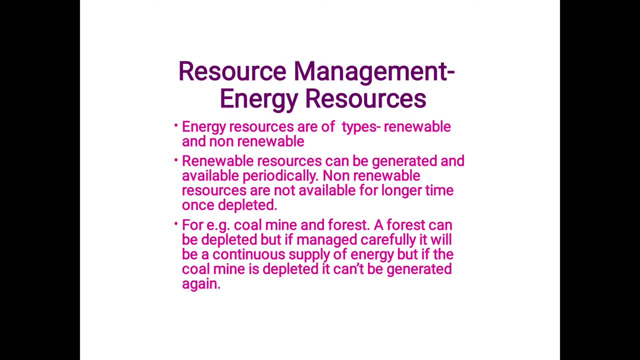 BSC 3, Semester 6.. Name of the paper: Environmental Geology. Name of the topic: Resource Management. Out of that we are going to learn energy resources. BSC 3, Semester 6.. Name of the paper: Environmental Geology. Name of the topic: Resource Management. Out of that we are going to learn energy resources. 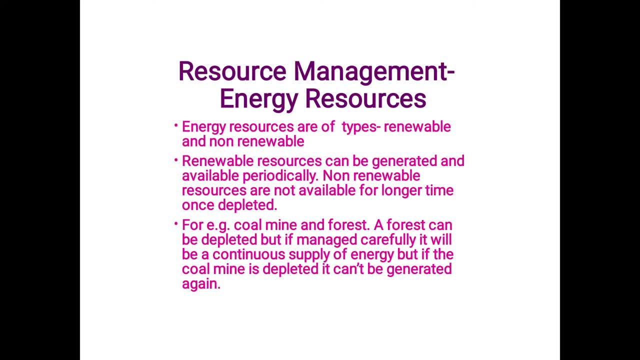 BSC 3, Semester 6.. Name of the paper: Environmental Geology. Name of the topic: Resource Management. Out of that we are going to learn energy resources. BSC 3, Semester 6.. Name of the paper: Environmental Geology. Name of the topic: Resource Management. Out of that we are going to learn energy resources. 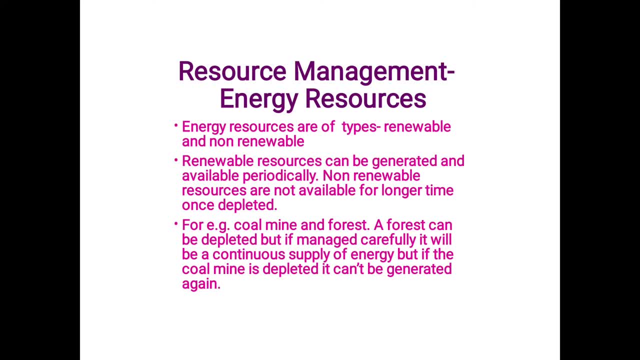 BSC 3, Semester 6.. Name of the paper: Environmental Geology. Name of the topic: Resource Management. Out of that we are going to learn energy resources. BSC 3, Semester 6.. Name of the paper: Environmental Geology. Name of the topic: Resource Management. Out of that we are going to learn energy resources. 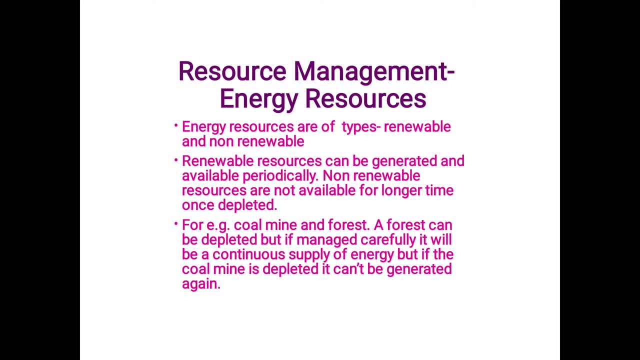 BSC 3, Semester 6.. Name of the paper: Environmental Geology. Name of the topic: Resource Management. Out of that we are going to learn energy resources. BSC 3, Semester 6.. Name of the paper: Environmental Geology. Name of the topic: Resource Management. Out of that we are going to learn energy resources. 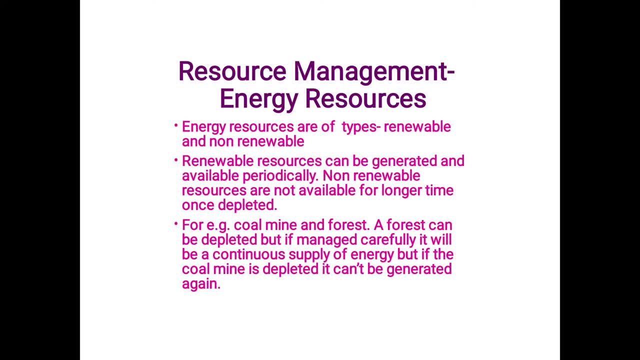 BSC 3, Semester 6.. Name of the paper: Environmental Geology. Name of the topic: Resource Management. Out of that we are going to learn energy resources. BSC 3, Semester 6.. Name of the paper: Environmental Geology. Name of the topic: Resource Management. Out of that we are going to learn energy resources. 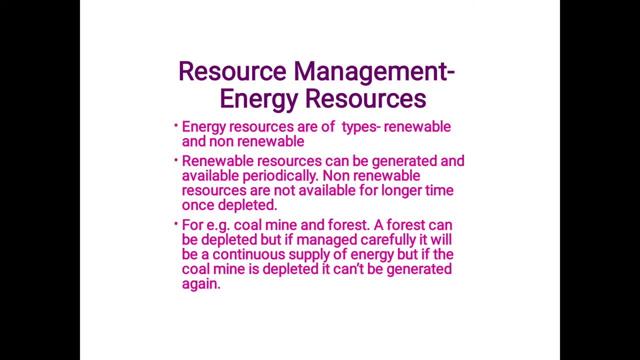 BSC 3, Semester 6.. Name of the paper: Environmental Geology. Name of the topic: Resource Management. Out of that we are going to learn energy resources. BSC 3, Semester 6.. Name of the paper: Environmental Geology. Name of the topic: Resource Management. Out of that we are going to learn energy resources. 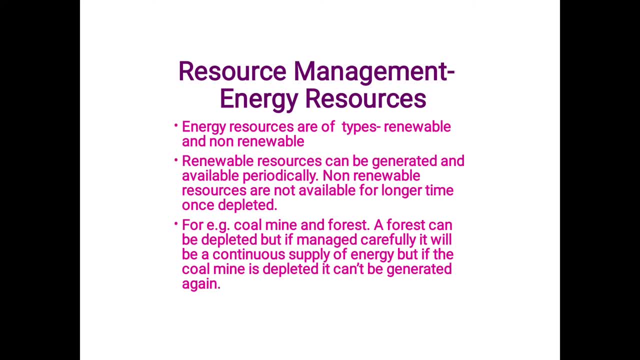 BSC 3, Semester 6.. Name of the paper: Environmental Geology. Name of the topic: Resource Management. Out of that we are going to learn energy resources. BSC 3, Semester 6.. Name of the paper: Environmental Geology. Name of the topic: Resource Management. Out of that we are going to learn energy resources. 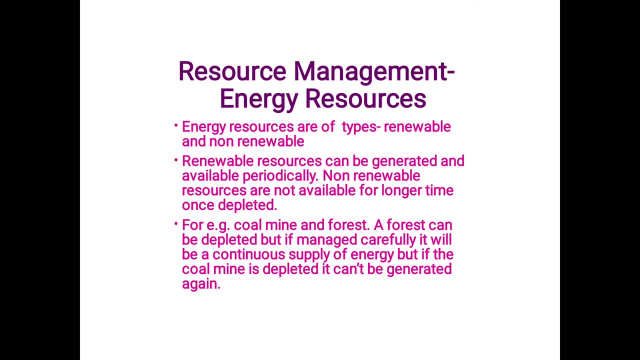 BSC 3, Semester 6.. Name of the paper: Environmental Geology. Name of the topic: Resource Management. Out of that we are going to learn energy resources. BSC 3, Semester 6.. Name of the paper: Environmental Geology. Name of the topic: Resource Management. Out of that we are going to learn energy resources. 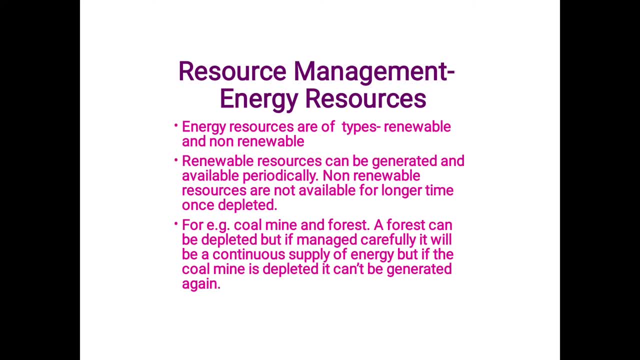 BSC 3, Semester 6.. Name of the paper: Environmental Geology. Name of the topic: Resource Management. Out of that we are going to learn energy resources. BSC 3, Semester 6.. Name of the paper: Environmental Geology. Name of the topic: Resource Management. Out of that we are going to learn energy resources. 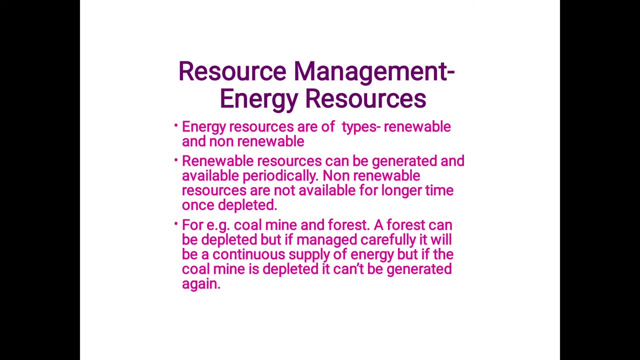 BSC 3, Semester 6.. Name of the paper: Environmental Geology. Name of the topic: Resource Management. Out of that we are going to learn energy resources. BSC 3, Semester 6.. Name of the paper: Environmental Geology. Name of the topic: Resource Management. Out of that we are going to learn energy resources. 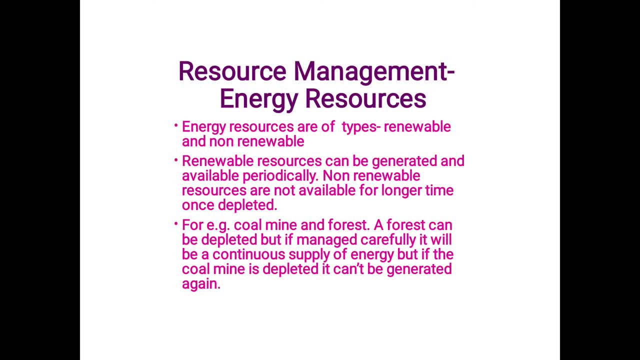 BSC 3, Semester 6.. Name of the paper: Environmental Geology. Name of the topic: Resource Management. Out of that we are going to learn energy resources. BSC 3, Semester 6.. Name of the paper: Environmental Geology. Name of the topic: Resource Management. Out of that we are going to learn energy resources. 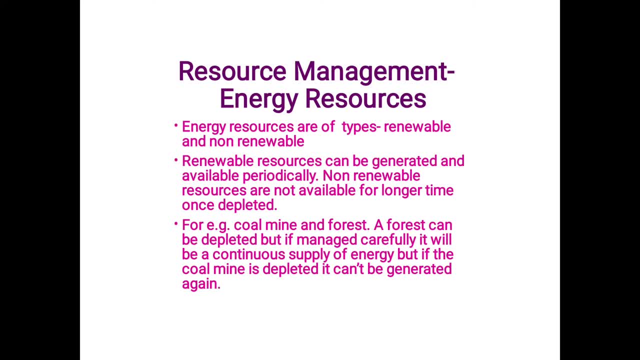 BSC 3, Semester 6.. Name of the paper: Environmental Geology. Name of the topic: Resource Management. Out of that we are going to learn energy resources. BSC 3, Semester 6.. Name of the paper: Environmental Geology. Name of the topic: Resource Management. Out of that we are going to learn energy resources. 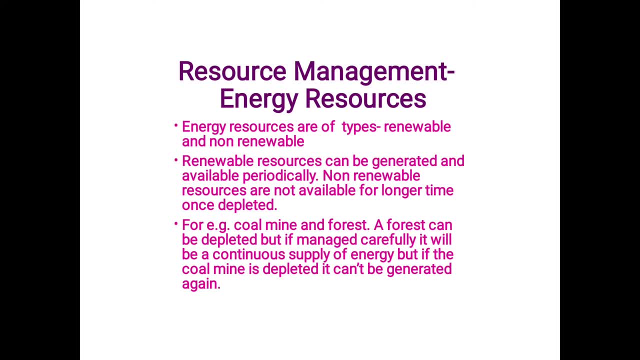 BSC 3, Semester 6.. Name of the paper: Environmental Geology. Name of the topic: Resource Management. Out of that we are going to learn energy resources. BSC 3, Semester 6.. Name of the paper: Environmental Geology. Name of the topic: Resource Management. Out of that we are going to learn energy resources. 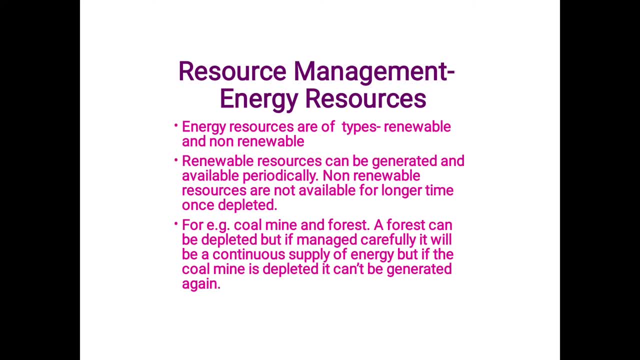 BSC 3, Semester 6.. Name of the paper: Environmental Geology. Name of the topic: Resource Management. Out of that we are going to learn energy resources. BSC 3, Semester 6.. Name of the paper: Environmental Geology. Name of the topic: Resource Management. Out of that we are going to learn energy resources. 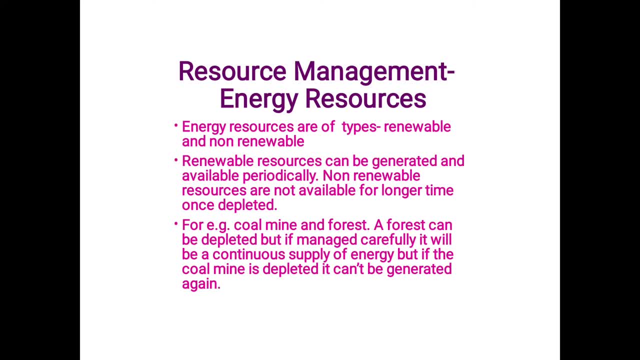 BSC 3, Semester 6.. Name of the paper: Environmental Geology. Name of the topic: Resource Management. Out of that we are going to learn energy resources. BSC 3, Semester 6.. Name of the paper: Environmental Geology. Name of the topic: Resource Management. Out of that we are going to learn energy resources. 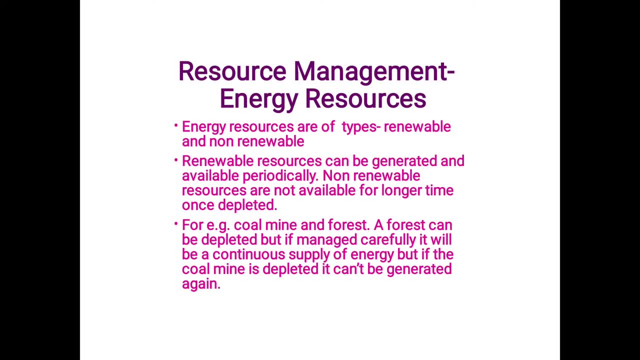 BSC 3, Semester 6.. Name of the paper: Environmental Geology. Name of the topic: Resource Management. Out of that we are going to learn energy resources. BSC 3, Semester 6.. Name of the paper: Environmental Geology. Name of the topic: Resource Management. Out of that we are going to learn energy resources. 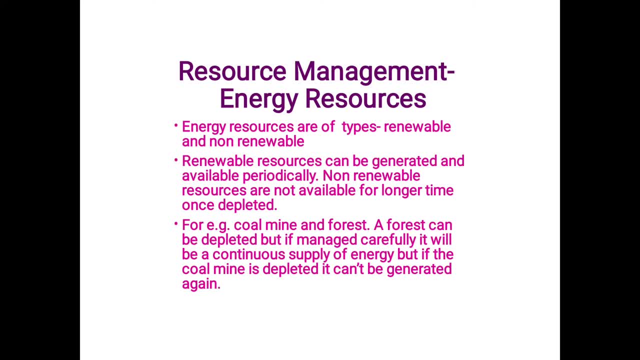 BSC 3, Semester 6.. Name of the paper: Environmental Geology. Name of the topic: Resource Management. Out of that we are going to learn energy resources. BSC 3, Semester 6.. Name of the paper: Environmental Geology. Name of the topic: Resource Management. Out of that we are going to learn energy resources. 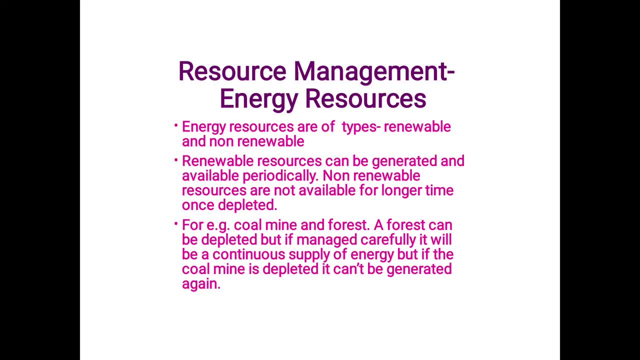 BSC 3, Semester 6.. Name of the paper: Environmental Geology. Name of the topic: Resource Management. Out of that we are going to learn energy resources. BSC 3, Semester 6.. Name of the paper: Environmental Geology. Name of the topic: Resource Management. Out of that we are going to learn energy resources. 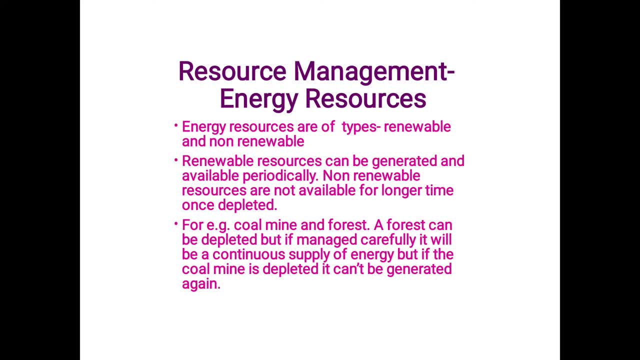 BSC 3, Semester 6.. Name of the paper: Environmental Geology. Name of the topic: Resource Management. Out of that we are going to learn energy resources. BSC 3, Semester 6.. Name of the paper: Environmental Geology. Name of the topic: Resource Management. Out of that we are going to learn energy resources. 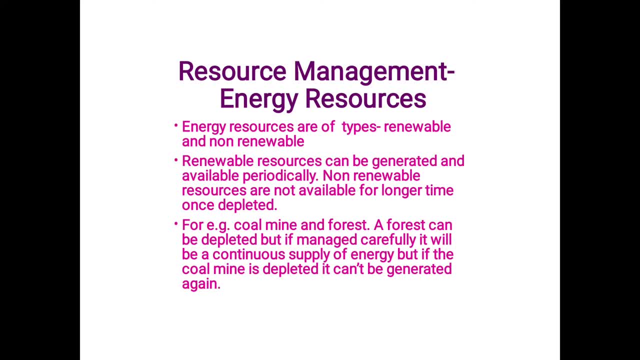 BSC 3, Semester 6.. Name of the paper: Environmental Geology. Name of the topic: Resource Management. Out of that we are going to learn energy resources. BSC 3, Semester 6.. Name of the paper: Environmental Geology. Name of the topic: Resource Management. Out of that we are going to learn energy resources. 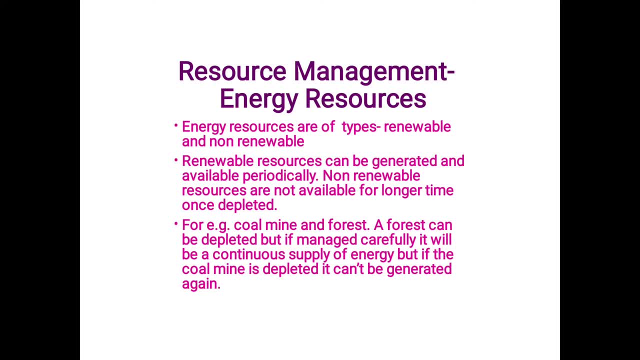 BSC 3, Semester 6.. Name of the paper: Environmental Geology. Name of the topic: Resource Management. Out of that we are going to learn energy resources. BSC 3, Semester 6.. Name of the paper: Environmental Geology. Name of the topic: Resource Management. Out of that we are going to learn energy resources. 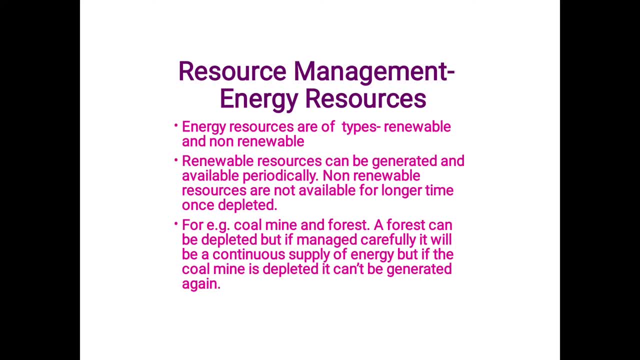 BSC 3, Semester 6.. Name of the paper: Environmental Geology. Name of the topic: Resource Management. Out of that we are going to learn energy resources. BSC 3, Semester 6.. Name of the paper: Environmental Geology. Name of the topic: Resource Management. Out of that we are going to learn energy resources. 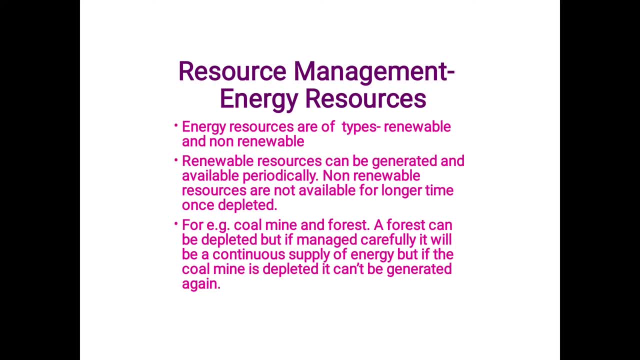 BSC 3, Semester 6.. Name of the paper: Environmental Geology. Name of the topic: Resource Management. Out of that we are going to learn energy resources. BSC 3, Semester 6.. Name of the paper: Environmental Geology. Name of the topic: Resource Management. Out of that we are going to learn energy resources. 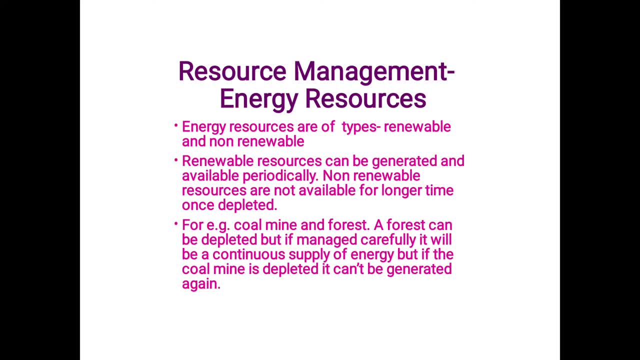 BSC 3, Semester 6.. Name of the paper: Environmental Geology. Name of the topic: Resource Management. Out of that we are going to learn energy resources. BSC 3, Semester 6.. Name of the paper: Environmental Geology. Name of the topic: Resource Management. Out of that we are going to learn energy resources. 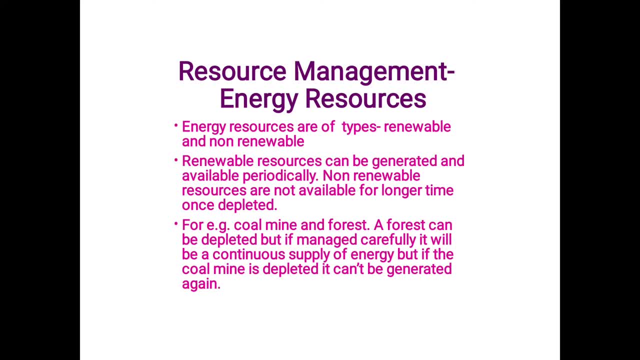 BSC 3, Semester 6.. Name of the paper: Environmental Geology. Name of the topic: Resource Management. Out of that we are going to learn energy resources. BSC 3, Semester 6.. Name of the paper: Environmental Geology. Name of the topic: Resource Management. Out of that we are going to learn energy resources. 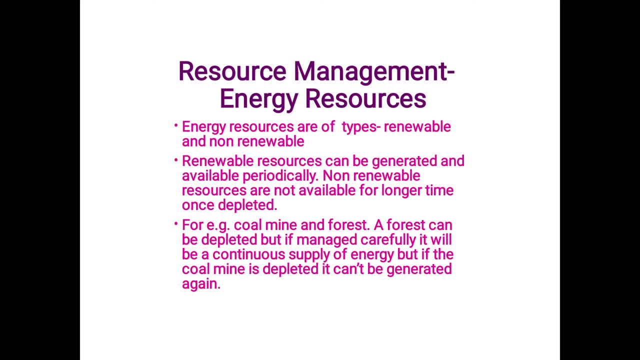 BSC 3, Semester 6.. Name of the paper: Environmental Geology. Name of the topic: Resource Management. Out of that we are going to learn energy resources. BSC 3, Semester 6.. Name of the paper: Environmental Geology. Name of the topic: Resource Management. Out of that we are going to learn energy resources. 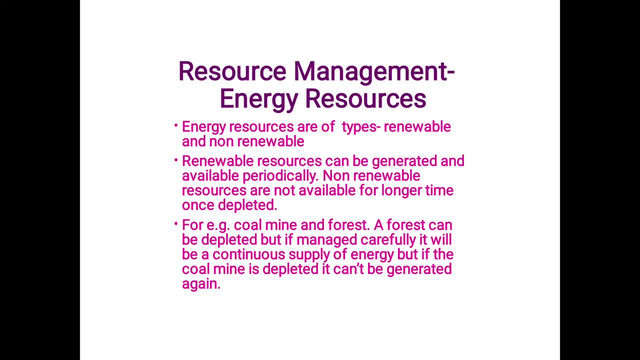 BSC 3, Semester 6.. Name of the paper: Environmental Geology. Name of the topic: Resource Management. Out of that we are going to learn energy resources. BSC 3, Semester 6.. Name of the paper: Environmental Geology. Name of the topic: Resource Management. Out of that we are going to learn energy resources. 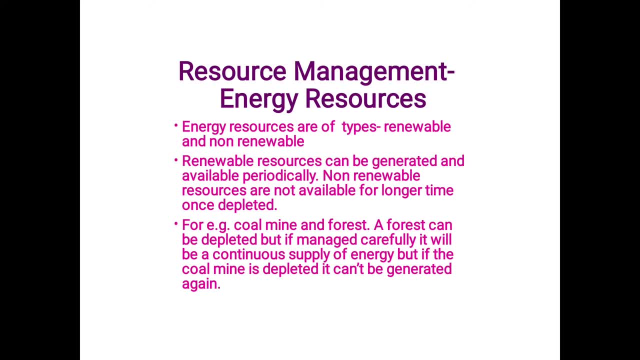 BSC 3, Semester 6.. Name of the paper: Environmental Geology. Name of the topic: Resource Management. Out of that we are going to learn energy resources. BSC 3, Semester 6.. Name of the paper: Environmental Geology. Name of the topic: Resource Management. Out of that we are going to learn energy resources. 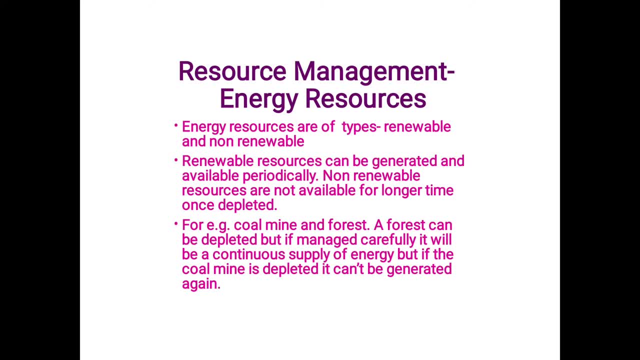 BSC 3, Semester 6.. Name of the paper: Environmental Geology. Name of the topic: Resource Management. Out of that we are going to learn energy resources. BSC 3, Semester 6.. Name of the paper: Environmental Geology. Name of the topic: Resource Management. Out of that we are going to learn energy resources. 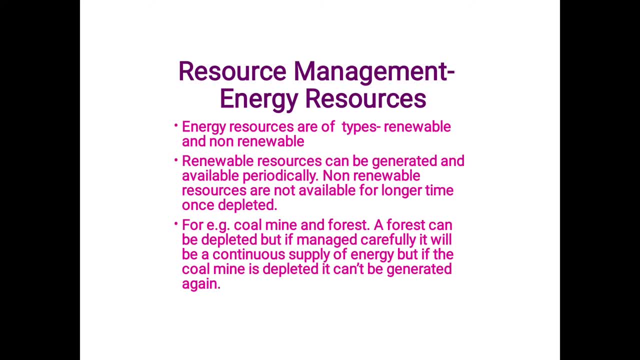 BSC 3, Semester 6.. Name of the paper: Environmental Geology. Name of the topic: Resource Management. Out of that we are going to learn energy resources. BSC 3, Semester 6.. Name of the paper: Environmental Geology. Name of the topic: Resource Management. Out of that we are going to learn energy resources. 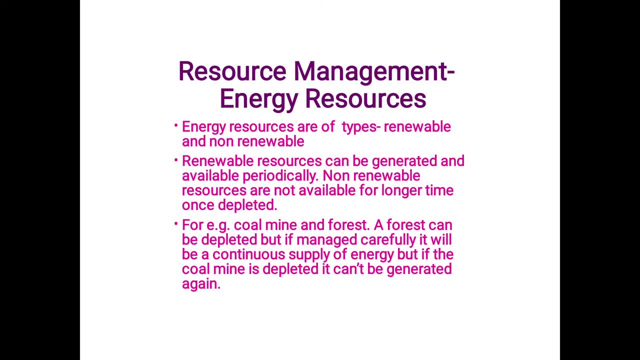 BSC 3, Semester 6.. Name of the paper: Environmental Geology. Name of the topic: Resource Management. Out of that we are going to learn energy resources. BSC 3, Semester 6.. Name of the paper: Environmental Geology. Name of the topic: Resource Management. Out of that we are going to learn energy resources. 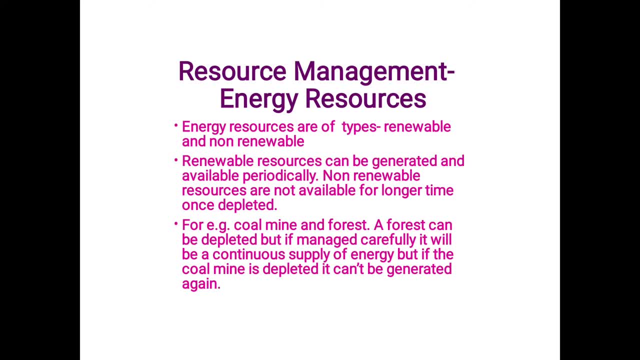 BSC 3, Semester 6.. Name of the paper: Environmental Geology. Name of the topic: Resource Management. Out of that we are going to learn energy resources. BSC 3, Semester 6.. Name of the paper: Environmental Geology. Name of the topic: Resource Management. Out of that we are going to learn energy resources. 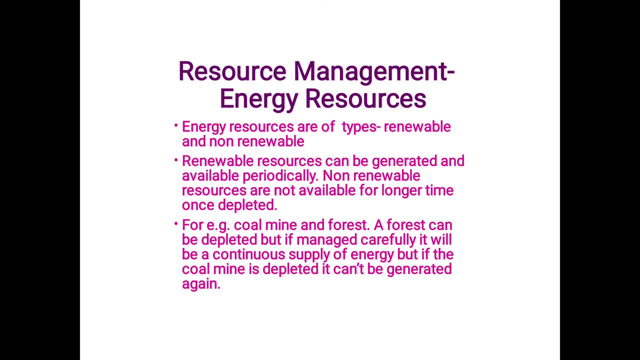 BSC 3, Semester 6.. Name of the paper: Environmental Geology. Name of the topic: Resource Management. Out of that we are going to learn energy resources. BSC 3, Semester 6.. Name of the paper: Environmental Geology. Name of the topic: Resource Management. Out of that we are going to learn energy resources. 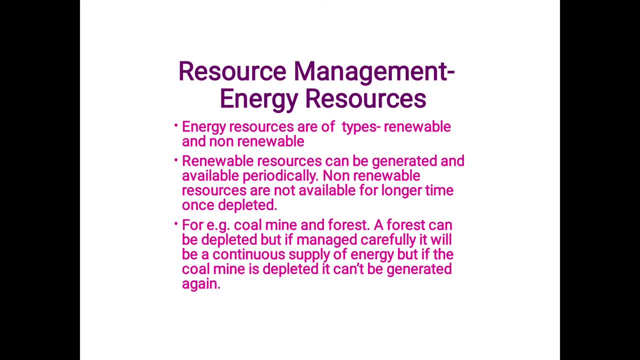 BSC 3, Semester 6.. Name of the paper: Environmental Geology. Name of the topic: Resource Management. Out of that we are going to learn energy resources. BSC 3, Semester 6.. Name of the paper: Environmental Geology. Name of the topic: Resource Management. Out of that we are going to learn energy resources. 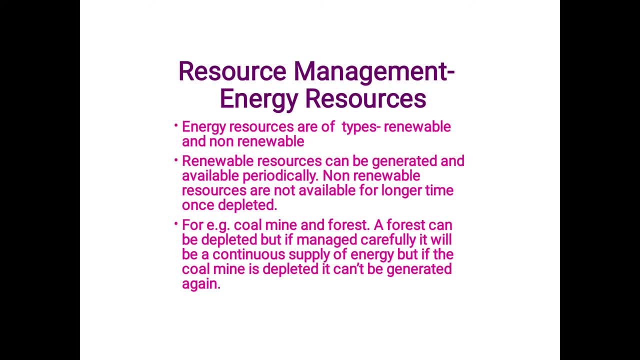 BSC 3, Semester 6.. Name of the paper: Environmental Geology. Name of the topic: Resource Management. Out of that we are going to learn energy resources. BSC 3, Semester 6.. Name of the paper: Environmental Geology. Name of the topic: Resource Management. Out of that we are going to learn energy resources. 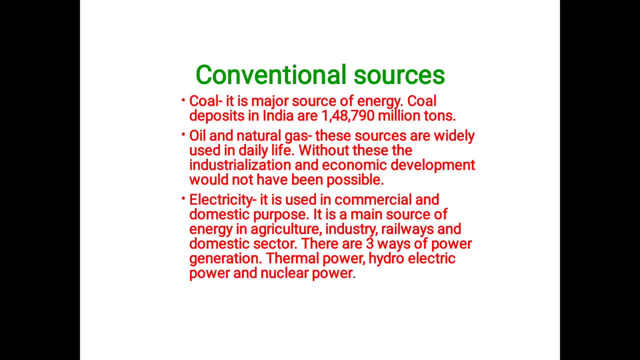 BSC 3, Semester 6.. Name of the paper: Environmental Geology. Name of the topic: Resource Management. Out of that we are going to learn energy resources. BSC 3, Semester 6.. Name of the paper: Environmental Geology. Name of the topic: Resource Management. Out of that we are going to learn energy resources. 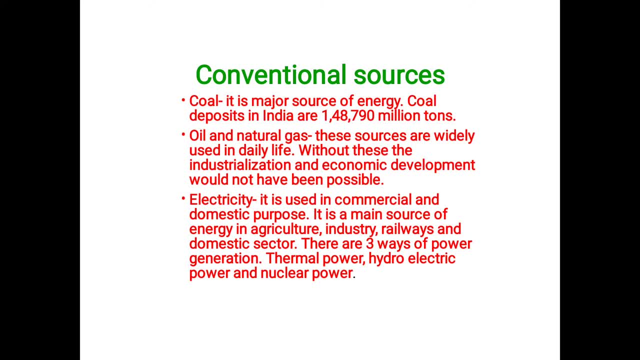 BSC 3, Semester 6.. Name of the paper: Environmental Geology. Name of the topic: Resource Management. Out of that we are going to learn energy resources. BSC 3, Semester 6.. Name of the paper: Environmental Geology. Name of the topic: Resource Management. Out of that we are going to learn energy resources. 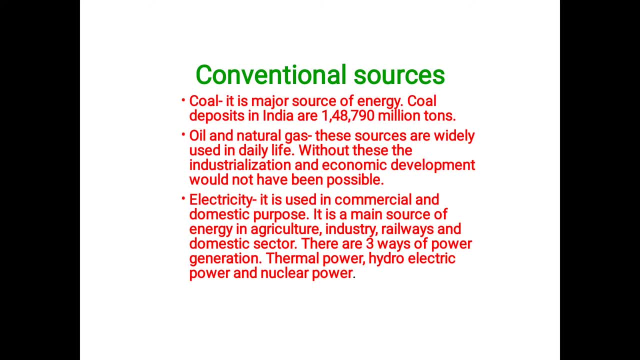 BSC 3, Semester 6.. Name of the paper: Environmental Geology. Name of the topic: Resource Management. Out of that we are going to learn energy resources. BSC 3, Semester 6.. Name of the paper: Environmental Geology. Name of the topic: Resource Management. Out of that we are going to learn energy resources. 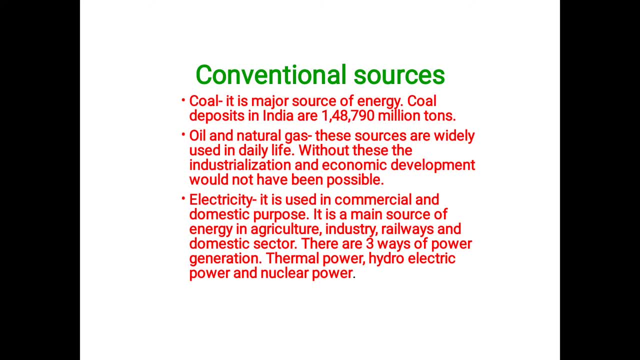 BSC 3, Semester 6.. Name of the paper: Environmental Geology. Name of the topic: Resource Management. Out of that we are going to learn energy resources. BSC 3, Semester 6.. Name of the paper: Environmental Geology. Name of the topic: Resource Management. Out of that we are going to learn energy resources. 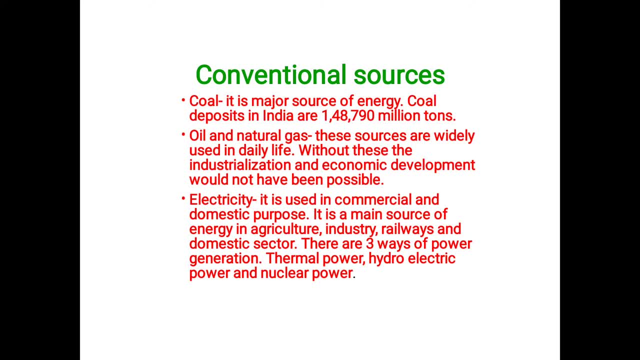 BSC 3, Semester 6.. Name of the paper: Environmental Geology. Name of the topic: Resource Management. Out of that we are going to learn energy resources. BSC 3, Semester 6.. Name of the paper: Environmental Geology. Name of the topic: Resource Management. Out of that we are going to learn energy resources. 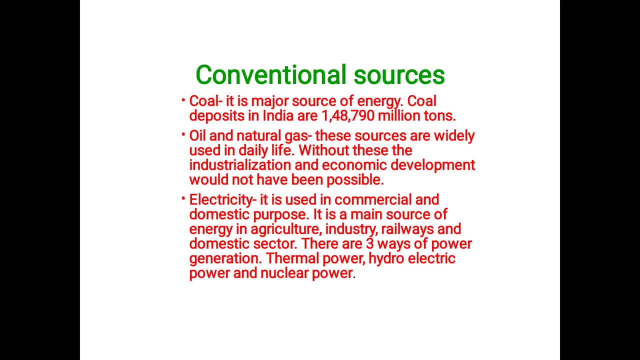 BSC 3, Semester 6.. Name of the paper: Environmental Geology. Name of the topic: Resource Management. Out of that we are going to learn energy resources. BSC 3, Semester 6.. Name of the paper: Environmental Geology. Name of the topic: Resource Management. Out of that we are going to learn energy resources. 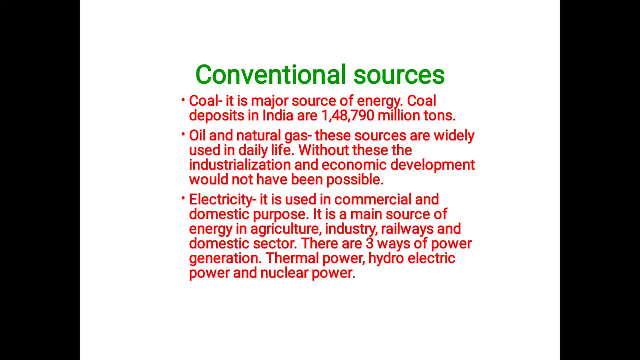 BSC 3, Semester 6.. Name of the paper: Environmental Geology. Name of the topic: Resource Management. Out of that we are going to learn energy resources. BSC 3, Semester 6.. Name of the paper: Environmental Geology. Name of the topic: Resource Management. Out of that we are going to learn energy resources. 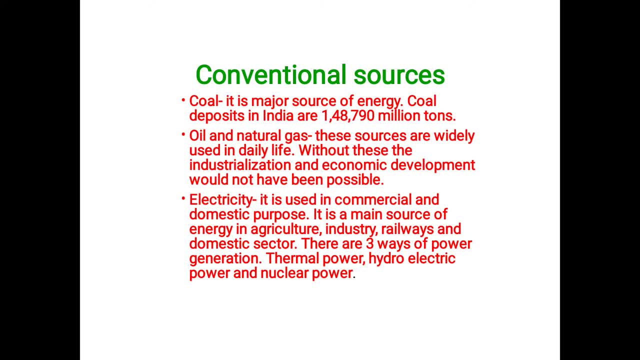 BSC 3, Semester 6.. Name of the paper: Environmental Geology. Name of the topic: Resource Management. Out of that we are going to learn energy resources. BSC 3, Semester 6.. Name of the paper: Environmental Geology. Name of the topic: Resource Management. Out of that we are going to learn energy resources. 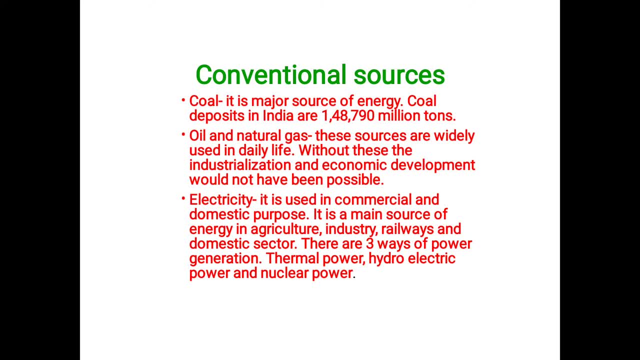 BSC 3, Semester 6.. Name of the paper: Environmental Geology. Name of the topic: Resource Management. Out of that we are going to learn energy resources. BSC 3, Semester 6.. Name of the paper: Environmental Geology. Name of the topic: Resource Management. Out of that we are going to learn energy resources. 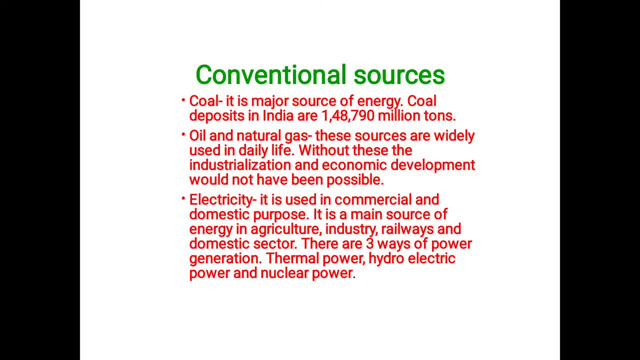 BSC 3, Semester 6.. Name of the paper: Environmental Geology. Name of the topic: Resource Management. Out of that we are going to learn energy resources. BSC 3, Semester 6.. Name of the paper: Environmental Geology. Name of the topic: Resource Management. Out of that we are going to learn energy resources. 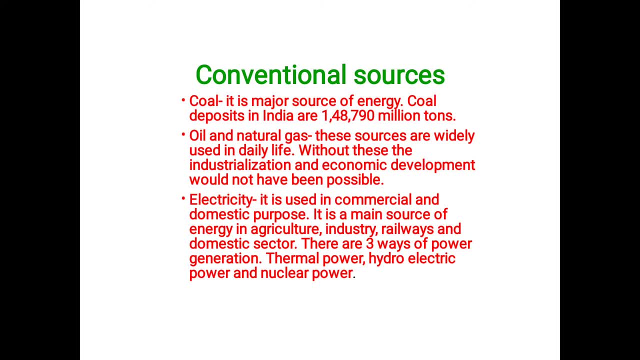 BSC 3, Semester 6.. Name of the paper: Environmental Geology. Name of the topic: Resource Management. Out of that we are going to learn energy resources. BSC 3, Semester 6.. Name of the paper: Environmental Geology. Name of the topic: Resource Management. Out of that we are going to learn energy resources. 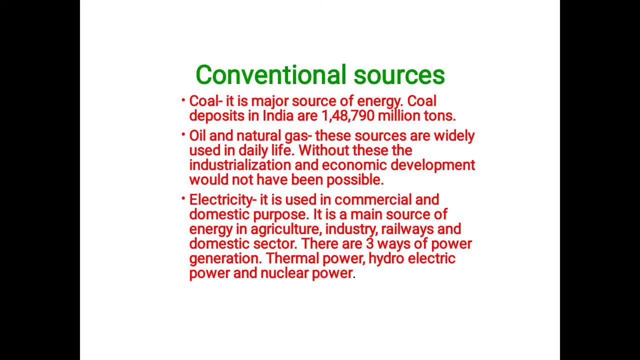 BSC 3, Semester 6.. Name of the paper: Environmental Geology. Name of the topic: Resource Management. Out of that we are going to learn energy resources. BSC 3, Semester 6.. Name of the paper: Environmental Geology. Name of the topic: Resource Management. Out of that we are going to learn energy resources. 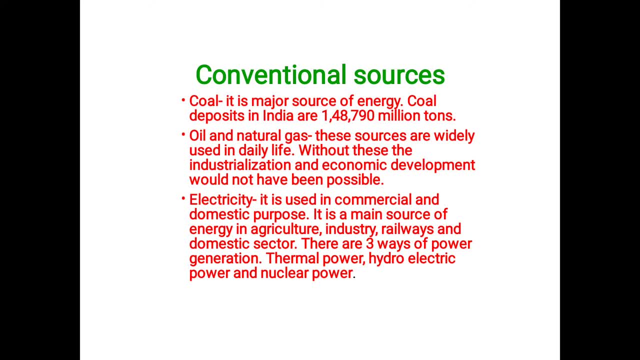 BSC 3, Semester 6.. Name of the paper: Environmental Geology. Name of the topic: Resource Management. Out of that we are going to learn energy resources. BSC 3, Semester 6.. Name of the paper: Environmental Geology. Name of the topic: Resource Management. Out of that we are going to learn energy resources. 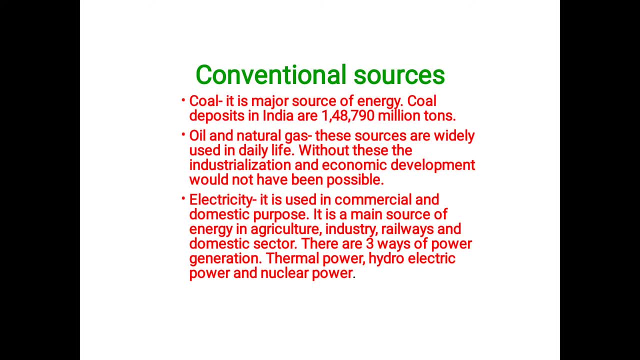 BSC 3, Semester 6.. Name of the paper: Environmental Geology. Name of the topic: Resource Management. Out of that we are going to learn energy resources. BSC 3, Semester 6.. Name of the paper: Environmental Geology. Name of the topic: Resource Management. Out of that we are going to learn energy resources. 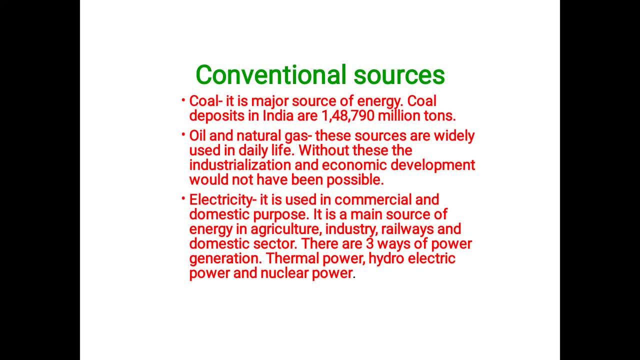 BSC 3, Semester 6.. Name of the paper: Environmental Geology. Name of the topic: Resource Management. Out of that we are going to learn energy resources. BSC 3, Semester 6.. Name of the paper: Environmental Geology. Name of the topic: Resource Management. Out of that we are going to learn energy resources. 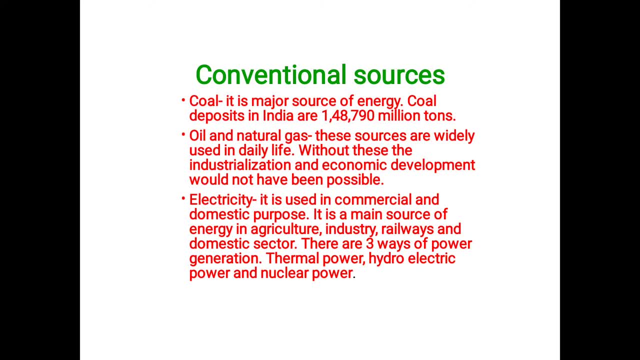 BSC 3, Semester 6.. Name of the paper: Environmental Geology. Name of the topic: Resource Management. Out of that we are going to learn energy resources. BSC 3, Semester 6.. Name of the paper: Environmental Geology. Name of the topic: Resource Management. Out of that we are going to learn energy resources. 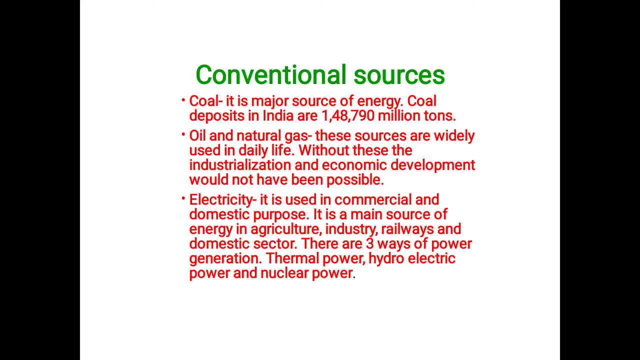 BSC 3, Semester 6.. Name of the paper: Environmental Geology. Name of the topic: Resource Management. Out of that we are going to learn energy resources. BSC 3, Semester 6.. Name of the paper: Environmental Geology. Name of the topic: Resource Management. Out of that we are going to learn energy resources. 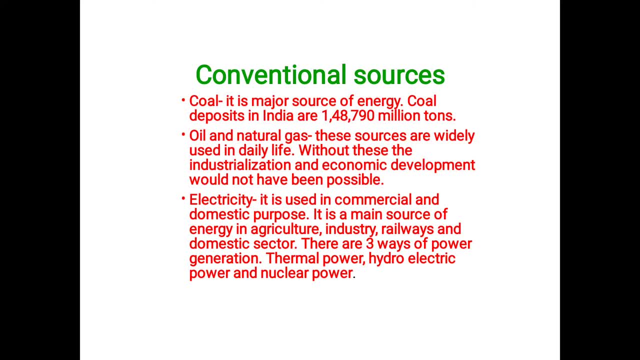 BSC 3, Semester 6.. Name of the paper: Environmental Geology. Name of the topic: Resource Management. Out of that we are going to learn energy resources. BSC 3, Semester 6.. Name of the paper: Environmental Geology. Name of the topic: Resource Management. Out of that we are going to learn energy resources. 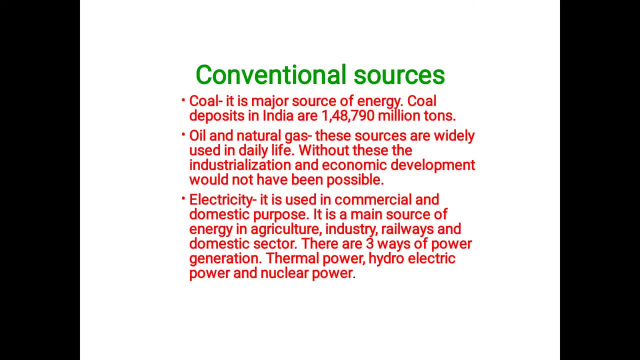 BSC 3, Semester 6.. Name of the paper: Environmental Geology. Name of the topic: Resource Management. Out of that we are going to learn energy resources. BSC 3, Semester 6.. Name of the paper: Environmental Geology. Name of the topic: Resource Management. Out of that we are going to learn energy resources. 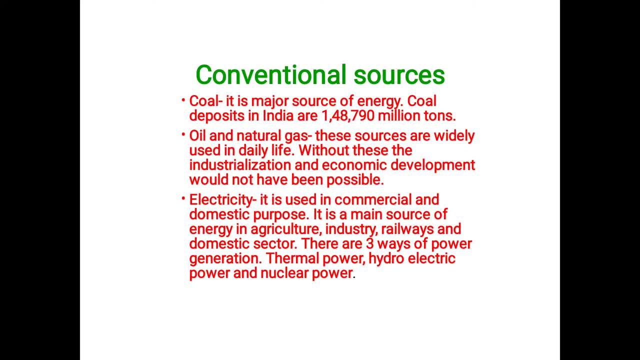 BSC 3, Semester 6.. Name of the paper: Environmental Geology. Name of the topic: Resource Management. Out of that we are going to learn energy resources. BSC 3, Semester 6.. Name of the paper: Environmental Geology. Name of the topic: Resource Management. Out of that we are going to learn energy resources. 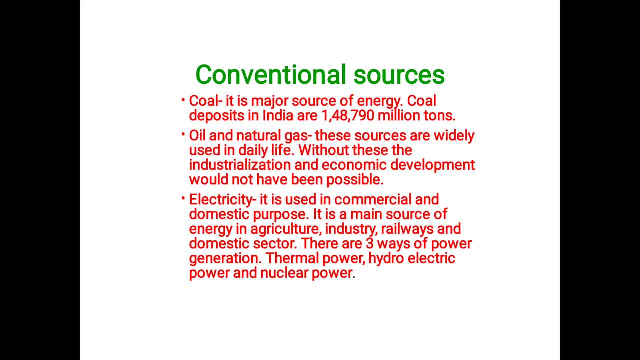 BSC 3, Semester 6.. Name of the paper: Environmental Geology. Name of the topic: Resource Management. Out of that we are going to learn energy resources. BSC 3, Semester 6.. Name of the paper: Environmental Geology. Name of the topic: Resource Management. Out of that we are going to learn energy resources. 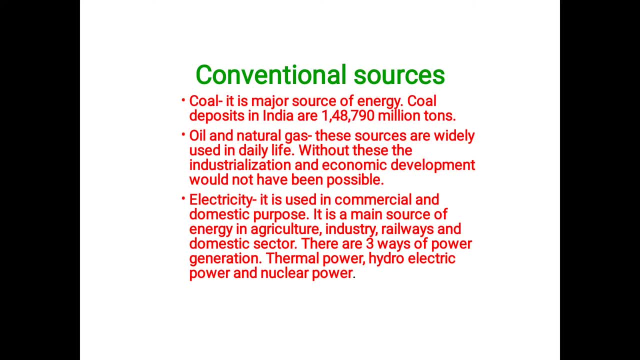 BSC 3, Semester 6.. Name of the paper: Environmental Geology. Name of the topic: Resource Management. Out of that we are going to learn energy resources. BSC 3, Semester 6.. Name of the paper: Environmental Geology. Name of the topic: Resource Management. Out of that we are going to learn energy resources. 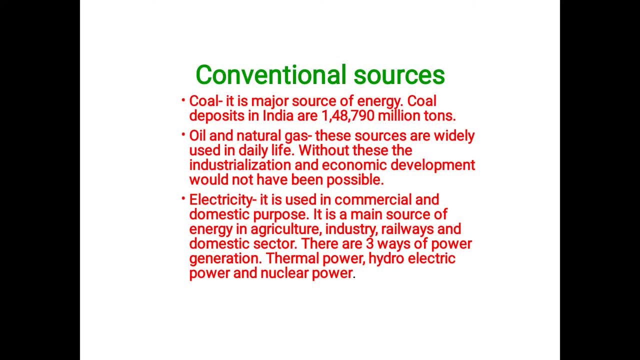 BSC 3, Semester 6.. Name of the paper: Environmental Geology. Name of the topic: Resource Management. Out of that we are going to learn energy resources. BSC 3, Semester 6.. Name of the paper: Environmental Geology. Name of the topic: Resource Management. Out of that we are going to learn energy resources. 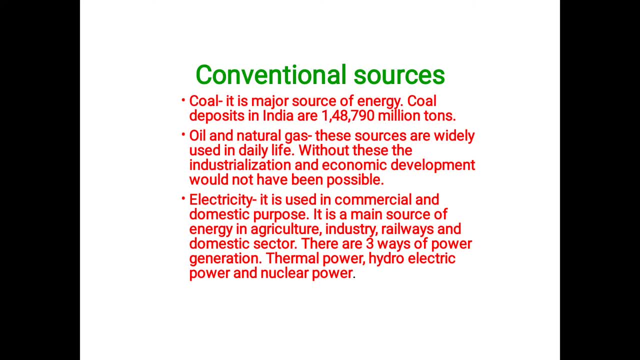 BSC 3, Semester 6.. Name of the paper: Environmental Geology. Name of the topic: Resource Management. Out of that we are going to learn energy resources. BSC 3, Semester 6.. Name of the paper: Environmental Geology. Name of the topic: Resource Management. Out of that we are going to learn energy resources. 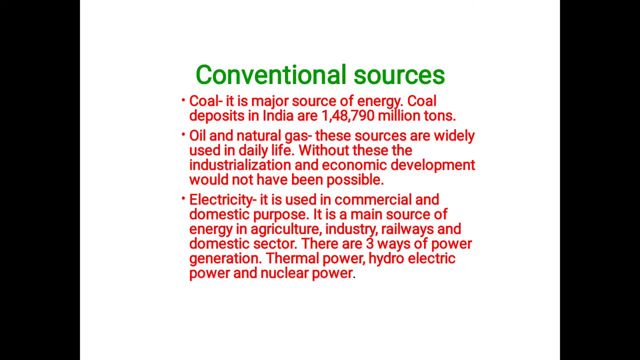 BSC 3, Semester 6.. Name of the paper: Environmental Geology. Name of the topic: Resource Management. Out of that we are going to learn energy resources. BSC 3, Semester 6.. Name of the paper: Environmental Geology. Name of the topic: Resource Management. Out of that we are going to learn energy resources. 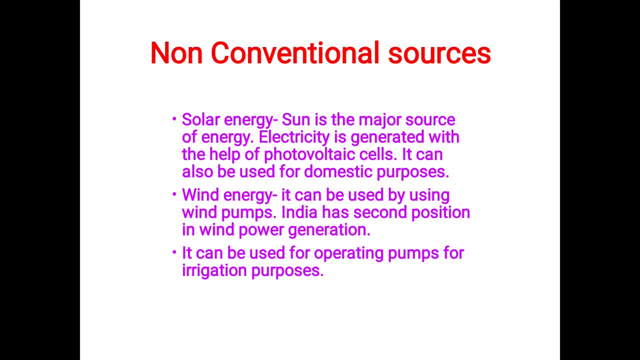 BSC 3, Semester 6.. Name of the paper: Environmental Geology. Name of the topic: Resource Management. Out of that we are going to learn energy resources. BSC 3, Semester 6.. Name of the paper: Environmental Geology. Name of the topic: Resource Management. Out of that we are going to learn energy resources. 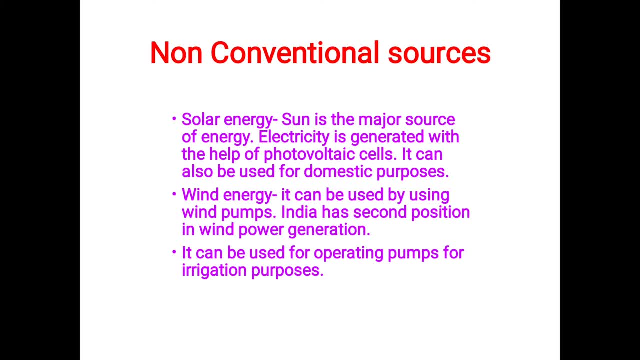 BSC 3, Semester 6.. Name of the paper: Environmental Geology. Name of the topic: Resource Management. Out of that we are going to learn energy resources. BSC 3, Semester 6.. Name of the paper: Environmental Geology. Name of the topic: Resource Management. Out of that we are going to learn energy resources. 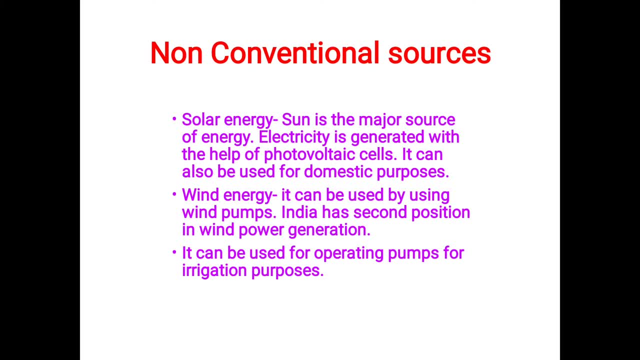 BSC 3, Semester 6.. Name of the paper: Environmental Geology. Name of the topic: Resource Management. Out of that we are going to learn energy resources. BSC 3, Semester 6.. Name of the paper: Environmental Geology. Name of the topic: Resource Management. Out of that we are going to learn energy resources. 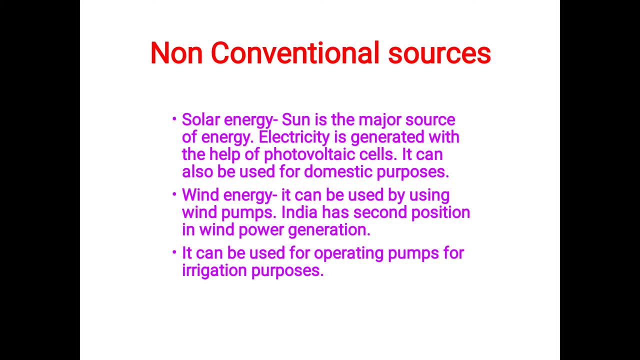 BSC 3, Semester 6.. Name of the paper: Environmental Geology. Name of the topic: Resource Management. Out of that we are going to learn energy resources. BSC 3, Semester 6.. Name of the paper: Environmental Geology. Name of the topic: Resource Management. Out of that we are going to learn energy resources. 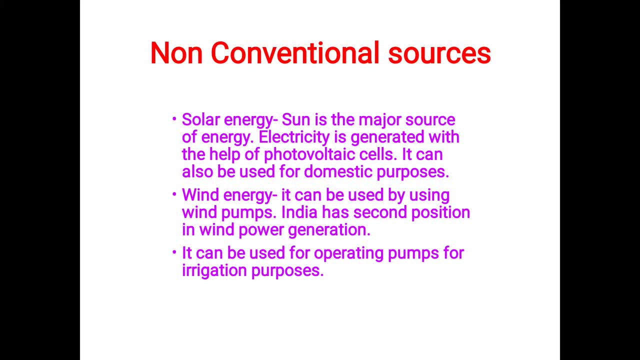 BSC 3, Semester 6.. Name of the paper: Environmental Geology. Name of the topic: Resource Management. Out of that we are going to learn energy resources. BSC 3, Semester 6.. Name of the paper: Environmental Geology. Name of the topic: Resource Management. Out of that we are going to learn energy resources. 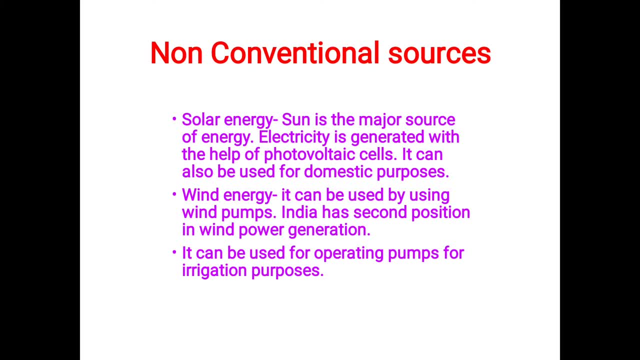 BSC 3, Semester 6.. Name of the paper: Environmental Geology. Name of the topic: Resource Management. Out of that we are going to learn energy resources. BSC 3, Semester 6.. Name of the paper: Environmental Geology. Name of the topic: Resource Management. Out of that we are going to learn energy resources. 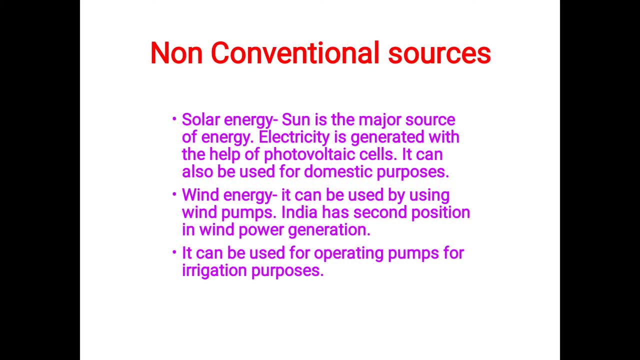 BSC 3, Semester 6.. Name of the paper: Environmental Geology. Name of the topic: Resource Management. Out of that we are going to learn energy resources. BSC 3, Semester 6.. Name of the paper: Environmental Geology. Name of the topic: Resource Management. Out of that we are going to learn energy resources. 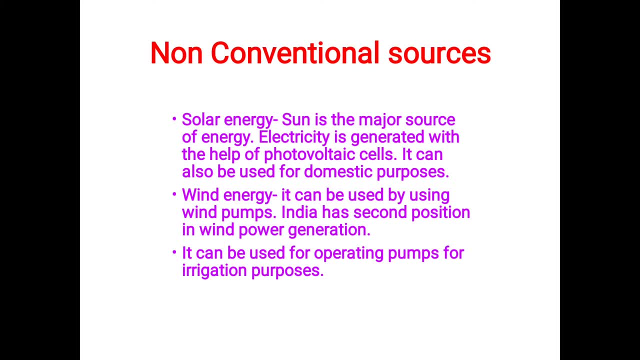 BSC 3, Semester 6.. Name of the paper: Environmental Geology. Name of the topic: Resource Management. Out of that we are going to learn energy resources. BSC 3, Semester 6.. Name of the paper: Environmental Geology. Name of the topic: Resource Management. Out of that we are going to learn energy resources. 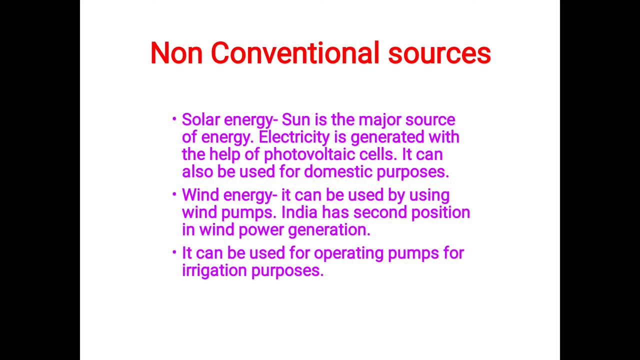 BSC 3, Semester 6.. Name of the paper: Environmental Geology. Name of the topic: Resource Management. Out of that we are going to learn energy resources. BSC 3, Semester 6.. Name of the paper: Environmental Geology. Name of the topic: Resource Management. Out of that we are going to learn energy resources. 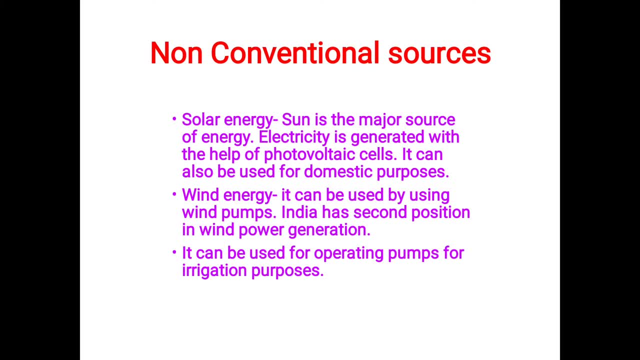 BSC 3, Semester 6.. Name of the paper: Environmental Geology. Name of the topic: Resource Management. Out of that we are going to learn energy resources. BSC 3, Semester 6.. Name of the paper: Environmental Geology. Name of the topic: Resource Management. Out of that we are going to learn energy resources. 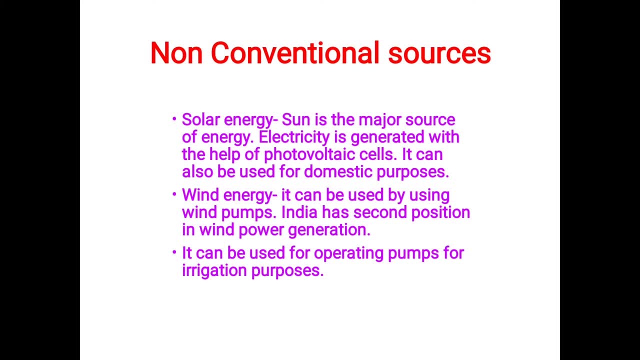 BSC 3, Semester 6.. Name of the paper: Environmental Geology. Name of the topic: Resource Management. Out of that we are going to learn energy resources. BSC 3, Semester 6.. Name of the paper: Environmental Geology. Name of the topic: Resource Management. Out of that we are going to learn energy resources. 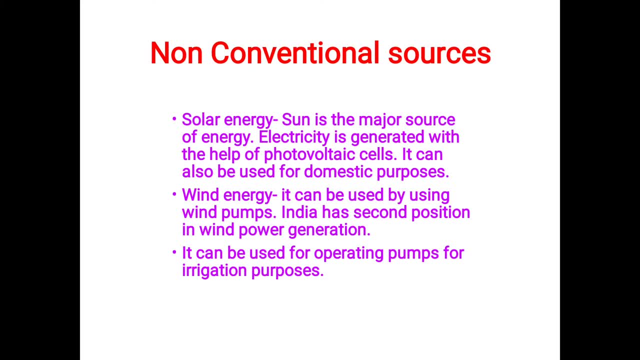 BSC 3, Semester 6.. Name of the paper: Environmental Geology. Name of the topic: Resource Management. Out of that we are going to learn energy resources. BSC 3, Semester 6.. Name of the paper: Environmental Geology. Name of the topic: Resource Management. Out of that we are going to learn energy resources. 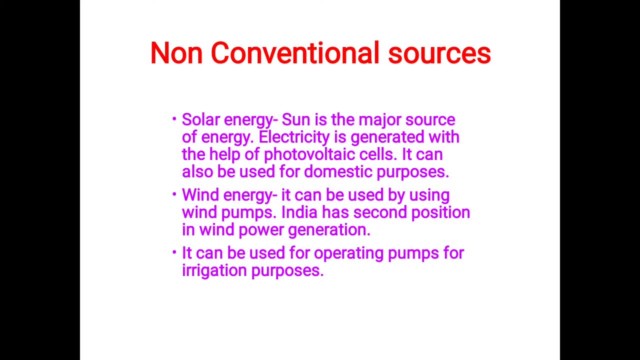 BSC 3, Semester 6.. Name of the paper: Environmental Geology. Name of the topic: Resource Management. Out of that we are going to learn energy resources. BSC 3, Semester 6.. Name of the paper: Environmental Geology. Name of the topic: Resource Management. Out of that we are going to learn energy resources. 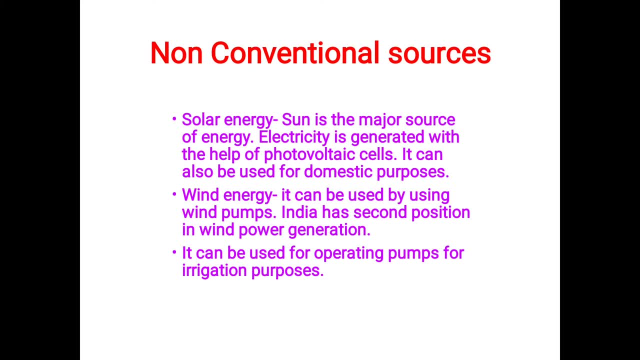 BSC 3, Semester 6.. Name of the paper: Environmental Geology. Name of the topic: Resource Management. Out of that we are going to learn energy resources. BSC 3, Semester 6.. Name of the paper: Environmental Geology. Name of the topic: Resource Management. Out of that we are going to learn energy resources. 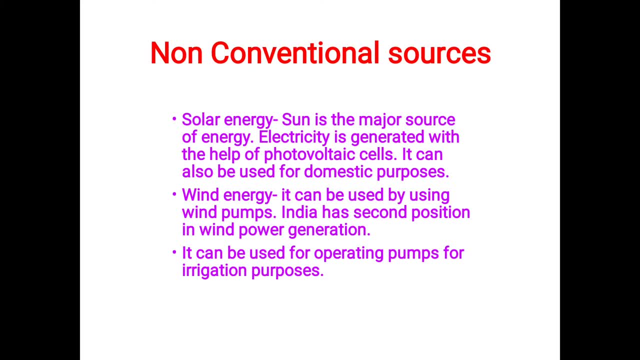 BSC 3, Semester 6.. Name of the paper: Environmental Geology. Name of the topic: Resource Management. Out of that we are going to learn energy resources. BSC 3, Semester 6.. Name of the paper: Environmental Geology. Name of the topic: Resource Management. Out of that we are going to learn energy resources. 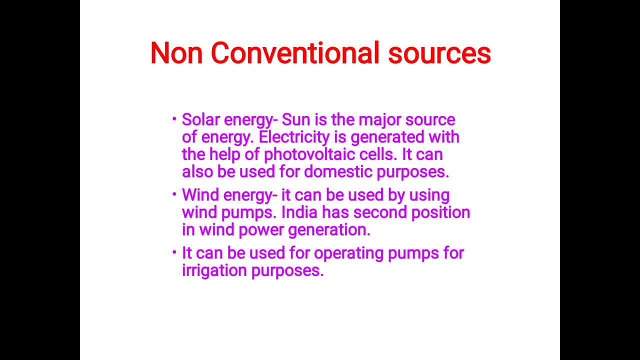 BSC 3, Semester 6.. Name of the paper: Environmental Geology. Name of the topic: Resource Management. Out of that we are going to learn energy resources. BSC 3, Semester 6.. Name of the paper: Environmental Geology. Name of the topic: Resource Management. Out of that we are going to learn energy resources. 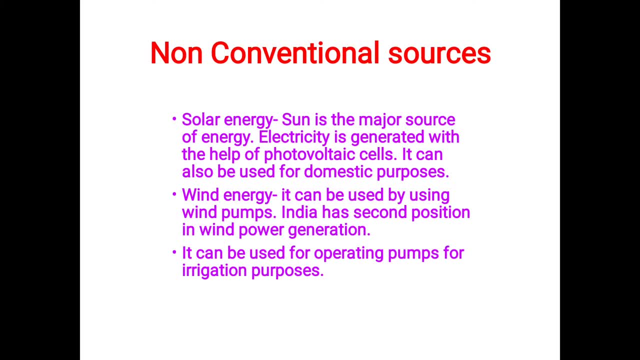 BSC 3, Semester 6.. Name of the paper: Environmental Geology. Name of the topic: Resource Management. Out of that we are going to learn energy resources. BSC 3, Semester 6.. Name of the paper: Environmental Geology. Name of the topic: Resource Management. Out of that we are going to learn energy resources. 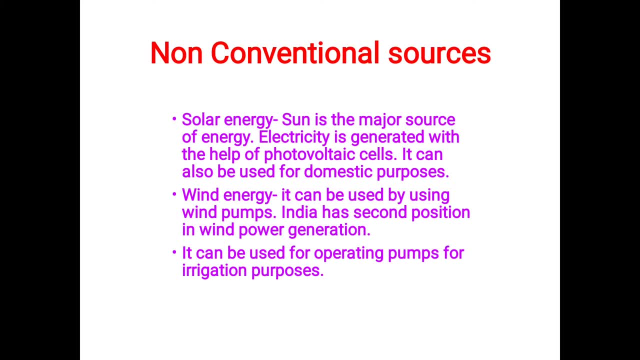 BSC 3, Semester 6.. Name of the paper: Environmental Geology. Name of the topic: Resource Management. Out of that we are going to learn energy resources. BSC 3, Semester 6.. Name of the paper: Environmental Geology. Name of the topic: Resource Management. Out of that we are going to learn energy resources. 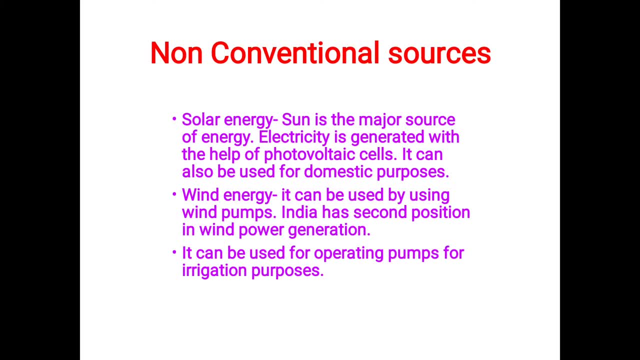 BSC 3, Semester 6.. Name of the paper: Environmental Geology. Name of the topic: Resource Management. Out of that we are going to learn energy resources. BSC 3, Semester 6.. Name of the paper: Environmental Geology. Name of the topic: Resource Management. Out of that we are going to learn energy resources. 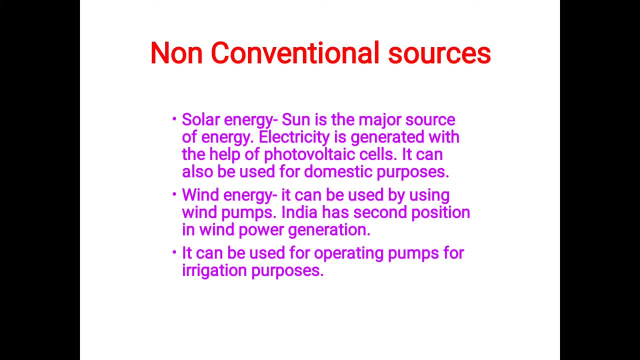 BSC 3, Semester 6.. Name of the paper: Environmental Geology. Name of the topic: Resource Management. Out of that we are going to learn energy resources. BSC 3, Semester 6.. Name of the paper: Environmental Geology. Name of the topic: Resource Management. Out of that we are going to learn energy resources. 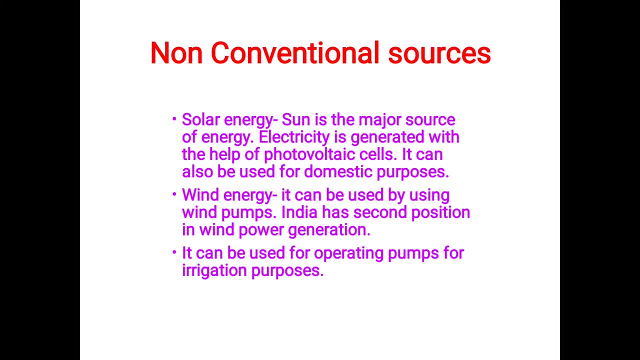 BSC 3, Semester 6.. Name of the paper: Environmental Geology. Name of the topic: Resource Management. Out of that we are going to learn energy resources. BSC 3, Semester 6.. Name of the paper: Environmental Geology. Name of the topic: Resource Management. Out of that we are going to learn energy resources. 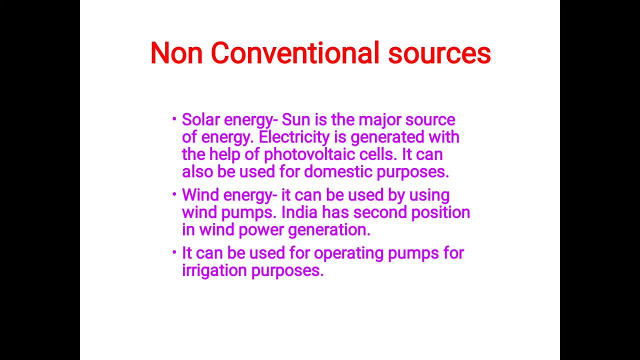 BSC 3, Semester 6.. Name of the paper: Environmental Geology. Name of the topic: Resource Management. Out of that we are going to learn energy resources. BSC 3, Semester 6.. Name of the paper: Environmental Geology. Name of the topic: Resource Management. Out of that we are going to learn energy resources. 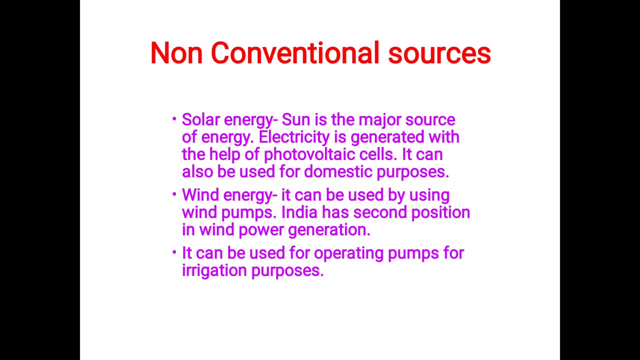 BSC 3, Semester 6.. Name of the paper: Environmental Geology. Name of the topic: Resource Management. Out of that we are going to learn energy resources. BSC 3, Semester 6.. Name of the paper: Environmental Geology. Name of the topic: Resource Management. Out of that we are going to learn energy resources. 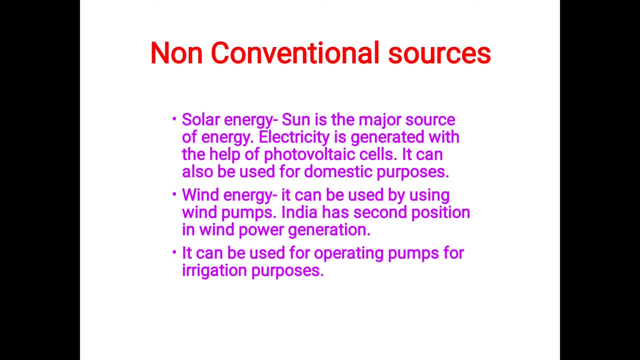 BSC 3, Semester 6.. Name of the paper: Environmental Geology. Name of the topic: Resource Management. Out of that we are going to learn energy resources. BSC 3, Semester 6.. Name of the paper: Environmental Geology. Name of the topic: Resource Management. Out of that we are going to learn energy resources. 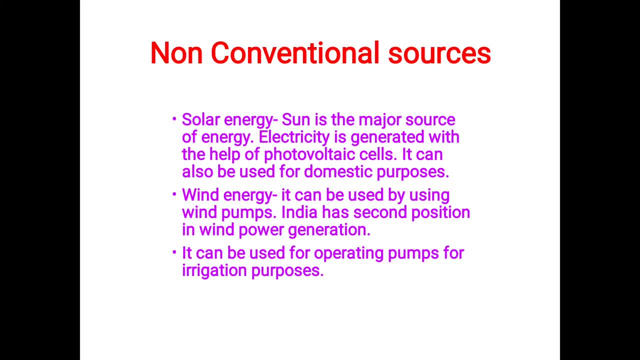 BSC 3, Semester 6.. Name of the paper: Environmental Geology. Name of the topic: Resource Management. Out of that we are going to learn energy resources. BSC 3, Semester 6.. Name of the paper: Environmental Geology. Name of the topic: Resource Management. Out of that we are going to learn energy resources. 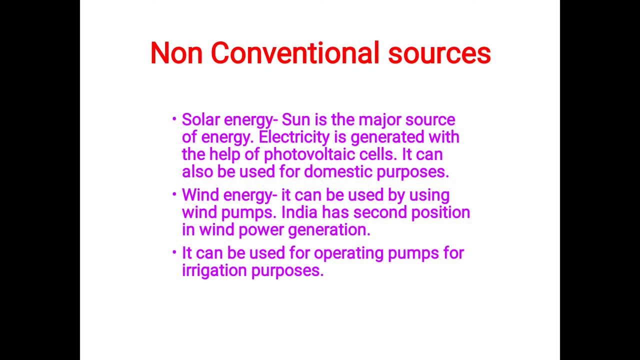 BSC 3, Semester 6.. Name of the paper: Environmental Geology. Name of the topic: Resource Management. Out of that we are going to learn energy resources. BSC 3, Semester 6.. Name of the paper: Environmental Geology. Name of the topic: Resource Management. Out of that we are going to learn energy resources. 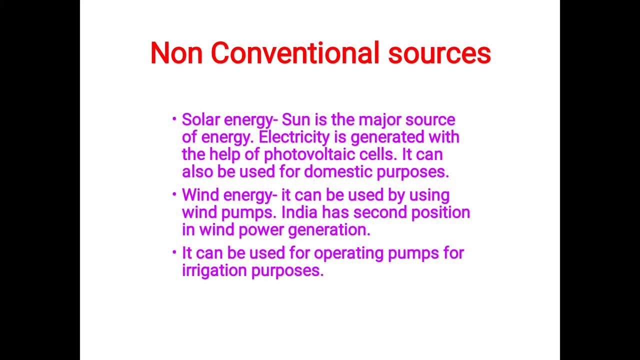 BSC 3, Semester 6.. Name of the paper: Environmental Geology. Name of the topic: Resource Management. Out of that we are going to learn energy resources. BSC 3, Semester 6.. Name of the paper: Environmental Geology. Name of the topic: Resource Management. Out of that we are going to learn energy resources. 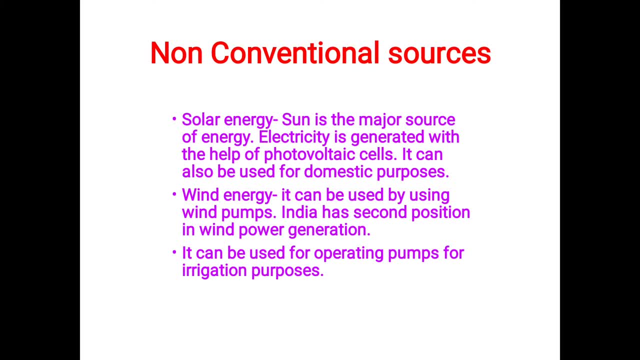 BSC 3, Semester 6.. Name of the paper: Environmental Geology. Name of the topic: Resource Management. Out of that we are going to learn energy resources. BSC 3, Semester 6.. Name of the paper: Environmental Geology. Name of the topic: Resource Management. Out of that we are going to learn energy resources. 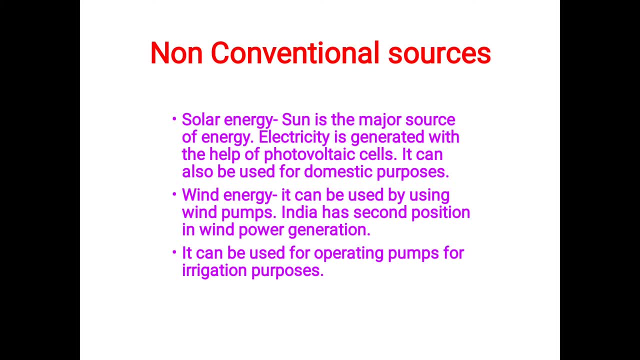 BSC 3, Semester 6.. Name of the paper: Environmental Geology. Name of the topic: Resource Management. Out of that we are going to learn energy resources. BSC 3, Semester 6.. Name of the paper: Environmental Geology. Name of the topic: Resource Management. Out of that we are going to learn energy resources. 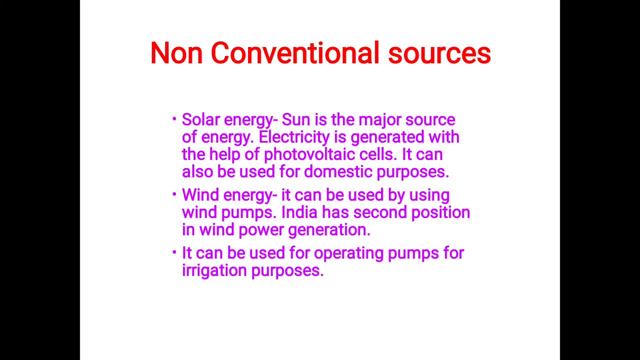 BSC 3, Semester 6.. Name of the paper: Environmental Geology. Name of the topic: Resource Management. Out of that we are going to learn energy resources. BSC 3, Semester 6.. Name of the paper: Environmental Geology. Name of the topic: Resource Management. Out of that we are going to learn energy resources. 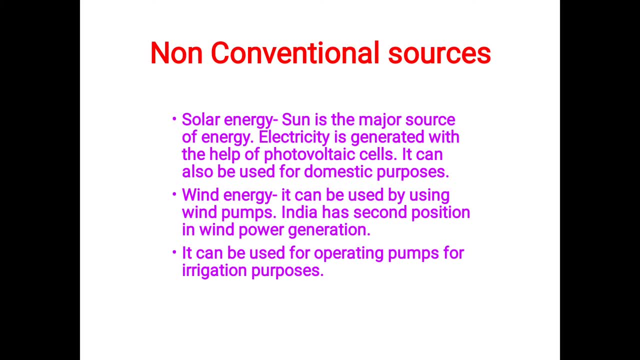 BSC 3, Semester 6.. Name of the paper: Environmental Geology. Name of the topic: Resource Management. Out of that we are going to learn energy resources. BSC 3, Semester 6.. Name of the paper: Environmental Geology. Name of the topic: Resource Management. Out of that we are going to learn energy resources. 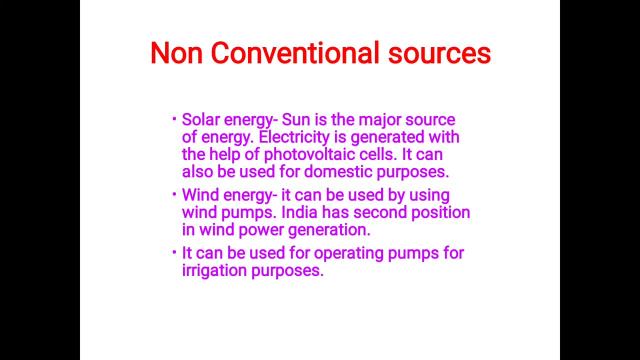 BSC 3, Semester 6.. Name of the paper: Environmental Geology. Name of the topic: Resource Management. Out of that we are going to learn energy resources. BSC 3, Semester 6.. Name of the paper: Environmental Geology. Name of the topic: Resource Management. Out of that we are going to learn energy resources. 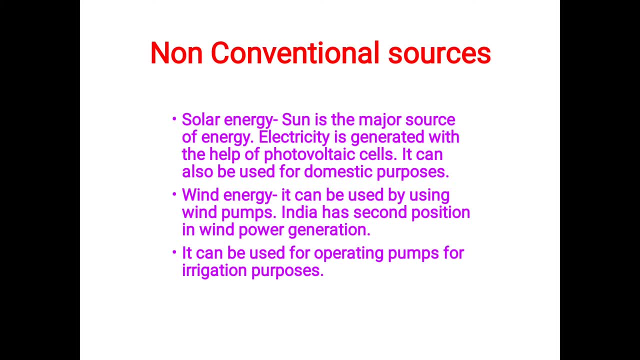 BSC 3, Semester 6.. Name of the paper: Environmental Geology. Name of the topic: Resource Management. Out of that we are going to learn energy resources. BSC 3, Semester 6.. Name of the paper: Environmental Geology. Name of the topic: Resource Management. Out of that we are going to learn energy resources. 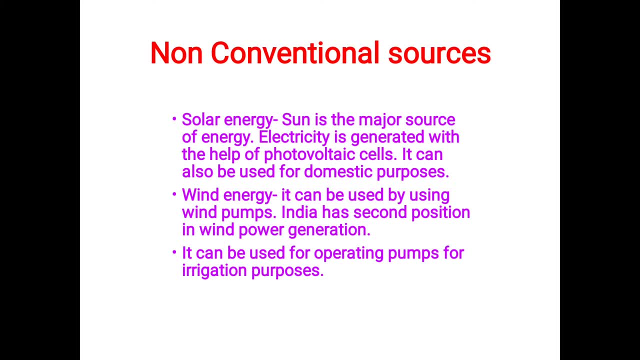 BSC 3, Semester 6.. Name of the paper: Environmental Geology. Name of the topic: Resource Management. Out of that we are going to learn energy resources. BSC 3, Semester 6.. Name of the paper: Environmental Geology. Name of the topic: Resource Management. Out of that we are going to learn energy resources. 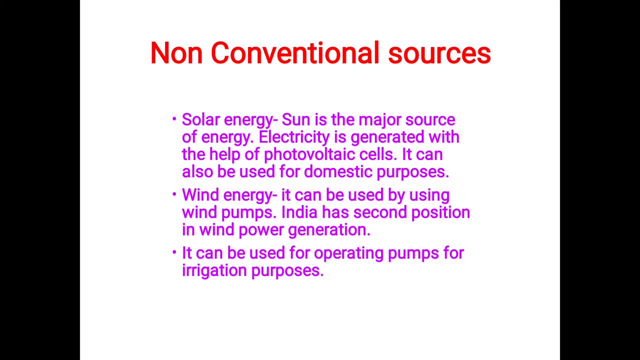 BSC 3, Semester 6.. Name of the paper: Environmental Geology. Name of the topic: Resource Management. Out of that we are going to learn energy resources. BSC 3, Semester 6.. Name of the paper: Environmental Geology. Name of the topic: Resource Management. Out of that we are going to learn energy resources. 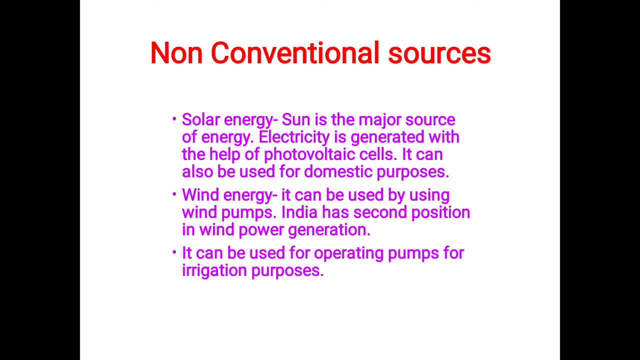 BSC 3, Semester 6.. Name of the paper: Environmental Geology. Name of the topic: Resource Management. Out of that we are going to learn energy resources. BSC 3, Semester 6.. Name of the paper: Environmental Geology. Name of the topic: Resource Management. Out of that we are going to learn energy resources. 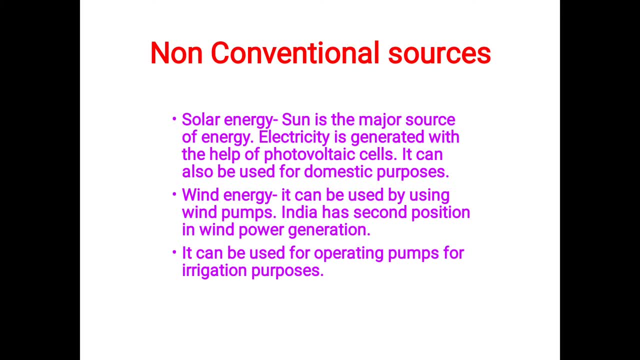 BSC 3, Semester 6.. Name of the paper: Environmental Geology. Name of the topic: Resource Management. Out of that we are going to learn energy resources. BSC 3, Semester 6.. Name of the paper: Environmental Geology. Name of the topic: Resource Management. Out of that we are going to learn energy resources. 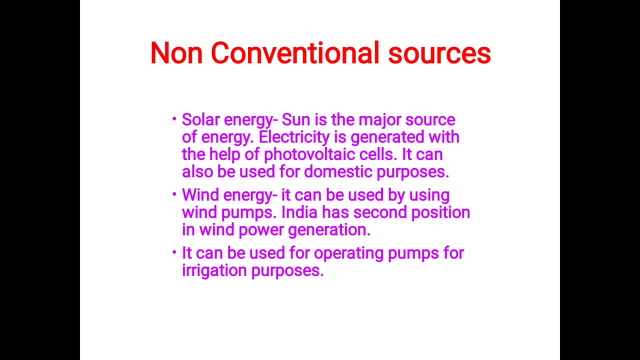 BSC 3, Semester 6.. Name of the paper: Environmental Geology. Name of the topic: Resource Management. Out of that we are going to learn energy resources. BSC 3, Semester 6.. Name of the paper: Environmental Geology. Name of the topic: Resource Management. Out of that we are going to learn energy resources. 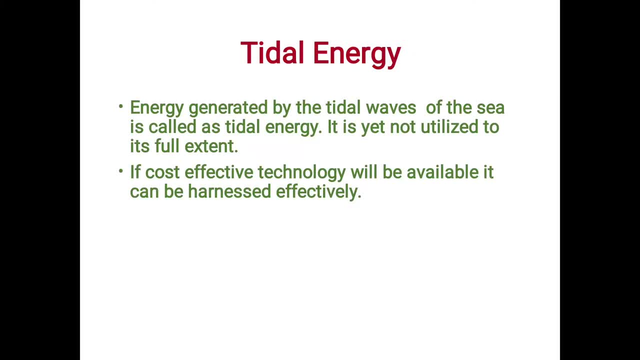 BSC 3, Semester 6.. Name of the paper: Environmental Geology. Name of the topic: Resource Management. Out of that we are going to learn energy resources. BSC 3, Semester 6.. Name of the paper: Environmental Geology. Name of the topic: Resource Management. Out of that we are going to learn energy resources. 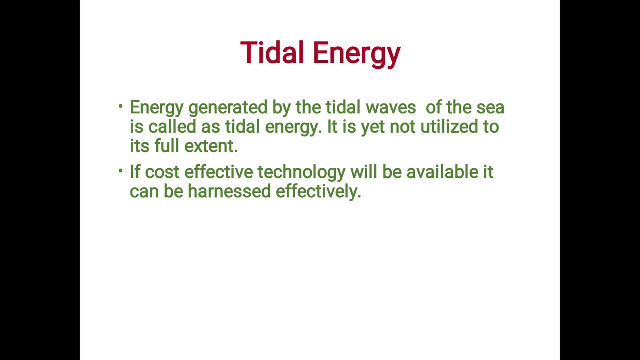 BSC 3, Semester 6.. Name of the paper: Environmental Geology. Name of the topic: Resource Management. Out of that we are going to learn energy resources. BSC 3, Semester 6.. Name of the paper: Environmental Geology. Name of the topic: Resource Management. Out of that we are going to learn energy resources. 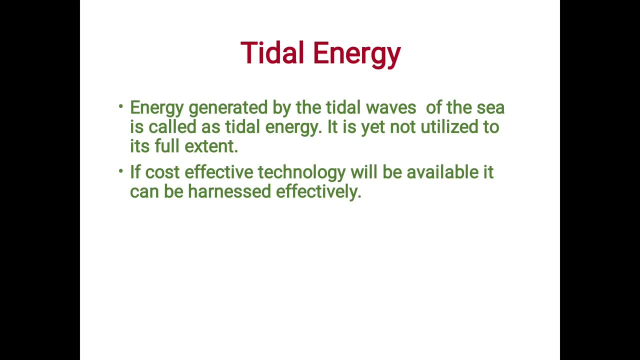 BSC 3, Semester 6.. Name of the paper: Environmental Geology. Name of the topic: Resource Management. Out of that we are going to learn energy resources. BSC 3, Semester 6.. Name of the paper: Environmental Geology. Name of the topic: Resource Management. Out of that we are going to learn energy resources. 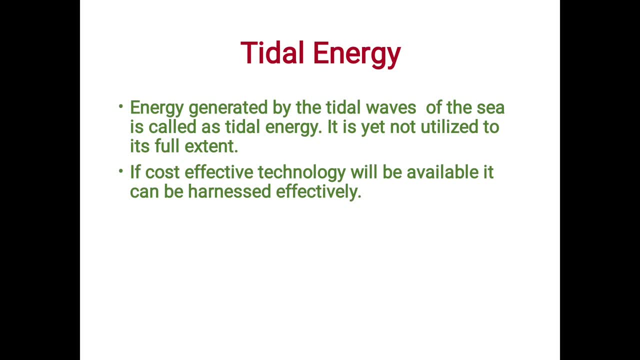 BSC 3, Semester 6.. Name of the paper: Environmental Geology. Name of the topic: Resource Management. Out of that we are going to learn energy resources. BSC 3, Semester 6.. Name of the paper: Environmental Geology. Name of the topic: Resource Management. Out of that we are going to learn energy resources. 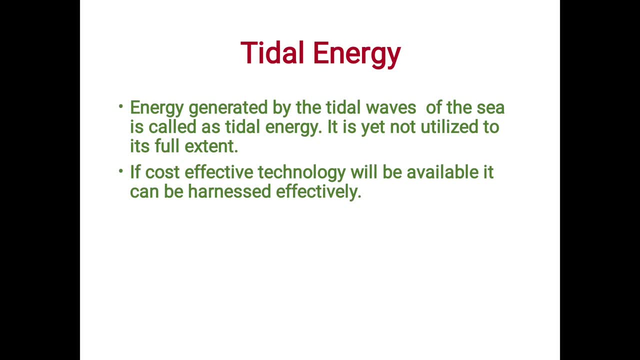 BSC 3, Semester 6.. Name of the paper: Environmental Geology. Name of the topic: Resource Management. Out of that we are going to learn energy resources. BSC 3, Semester 6.. Name of the paper: Environmental Geology. Name of the topic: Resource Management. Out of that we are going to learn energy resources. 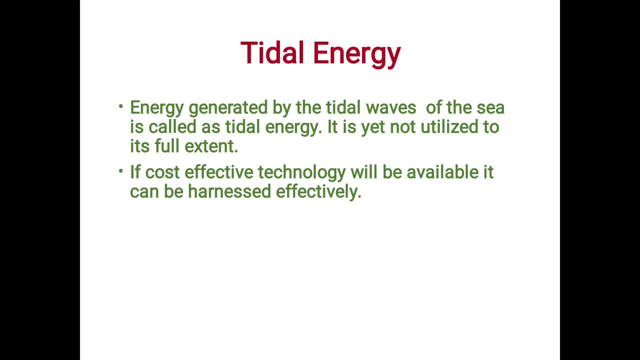 BSC 3, Semester 6.. Name of the paper: Environmental Geology. Name of the topic: Resource Management. Out of that we are going to learn energy resources. BSC 3, Semester 6.. Name of the paper: Environmental Geology. Name of the topic: Resource Management. Out of that we are going to learn energy resources. 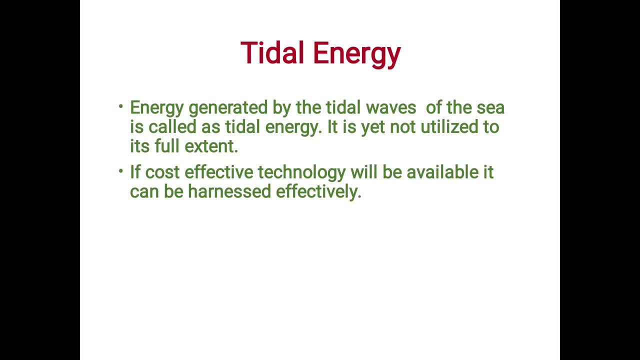 BSC 3, Semester 6.. Name of the paper: Environmental Geology. Name of the topic: Resource Management. Out of that we are going to learn energy resources. BSC 3, Semester 6.. Name of the paper: Environmental Geology. Name of the topic: Resource Management. Out of that we are going to learn energy resources. 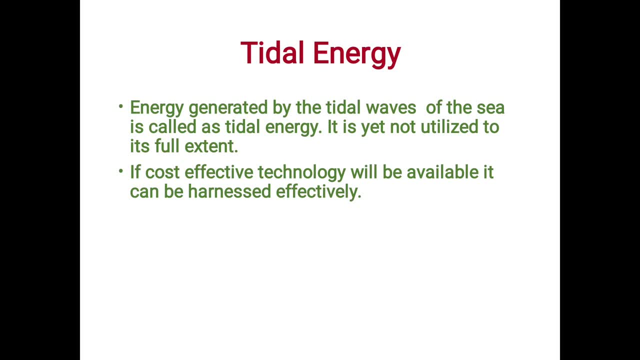 BSC 3, Semester 6.. Name of the paper: Environmental Geology. Name of the topic: Resource Management. Out of that we are going to learn energy resources. BSC 3, Semester 6.. Name of the paper: Environmental Geology. Name of the topic: Resource Management. Out of that we are going to learn energy resources. 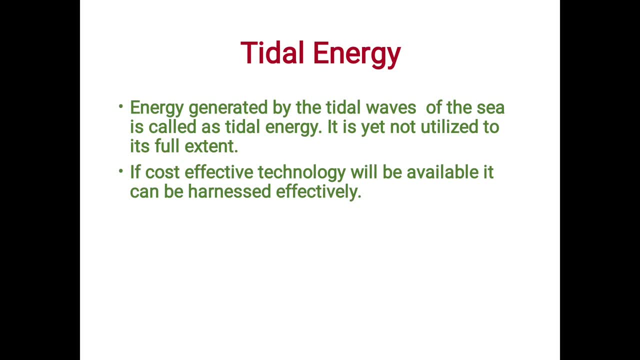 BSC 3, Semester 6.. Name of the paper: Environmental Geology. Name of the topic: Resource Management. Out of that we are going to learn energy resources. BSC 3, Semester 6.. Name of the paper: Environmental Geology. Name of the topic: Resource Management. Out of that we are going to learn energy resources. 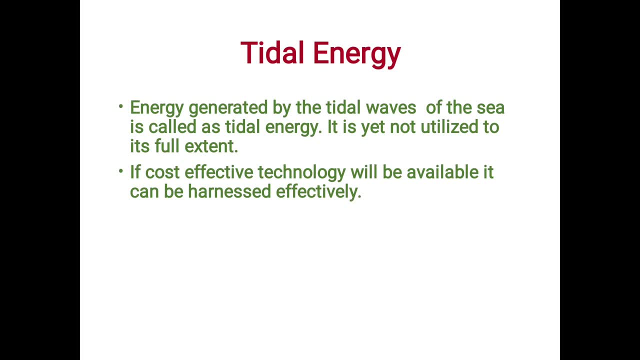 BSC 3, Semester 6.. Name of the paper: Environmental Geology. Name of the topic: Resource Management. Out of that we are going to learn energy resources. BSC 3, Semester 6.. Name of the paper: Environmental Geology. Name of the topic: Resource Management. Out of that we are going to learn energy resources. 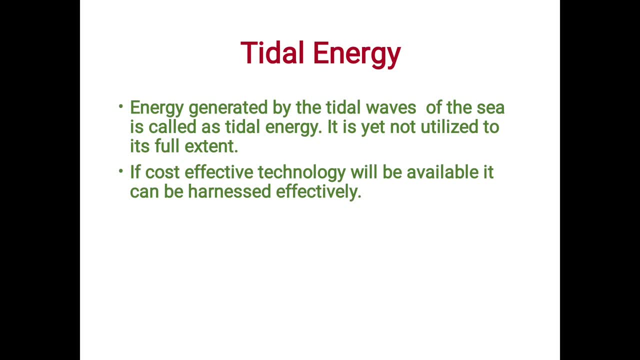 BSC 3, Semester 6.. Name of the paper: Environmental Geology. Name of the topic: Resource Management. Out of that we are going to learn energy resources. BSC 3, Semester 6.. Name of the paper: Environmental Geology. Name of the topic: Resource Management. Out of that we are going to learn energy resources. 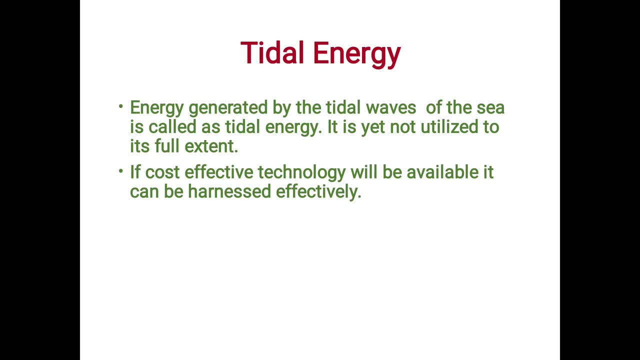 BSC 3, Semester 6.. Name of the paper: Environmental Geology. Name of the topic: Resource Management. Out of that we are going to learn energy resources. BSC 3, Semester 6.. Name of the paper: Environmental Geology. Name of the topic: Resource Management. Out of that we are going to learn energy resources. 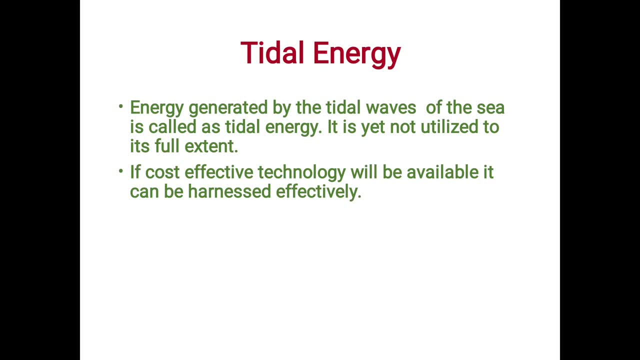 BSC 3, Semester 6.. Name of the paper: Environmental Geology. Name of the topic: Resource Management. Out of that we are going to learn energy resources. BSC 3, Semester 6.. Name of the paper: Environmental Geology. Name of the topic: Resource Management. Out of that we are going to learn energy resources. 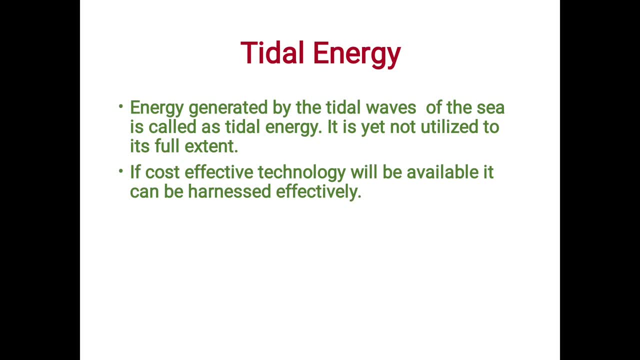 BSC 3, Semester 6.. Name of the paper: Environmental Geology. Name of the topic: Resource Management. Out of that we are going to learn energy resources. BSC 3, Semester 6.. Name of the paper: Environmental Geology. Name of the topic: Resource Management. Out of that we are going to learn energy resources. 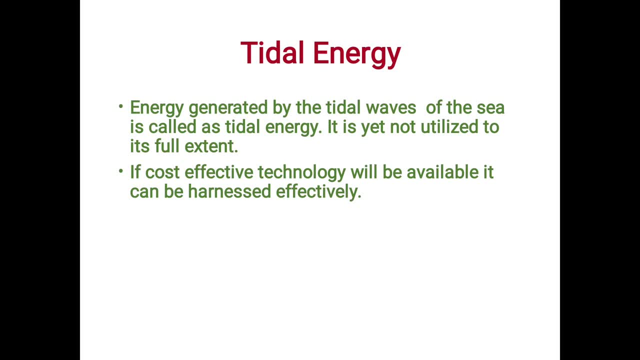 BSC 3, Semester 6.. Name of the paper: Environmental Geology. Name of the topic: Resource Management. Out of that we are going to learn energy resources. BSC 3, Semester 6.. Name of the paper: Environmental Geology. Name of the topic: Resource Management. Out of that we are going to learn energy resources. 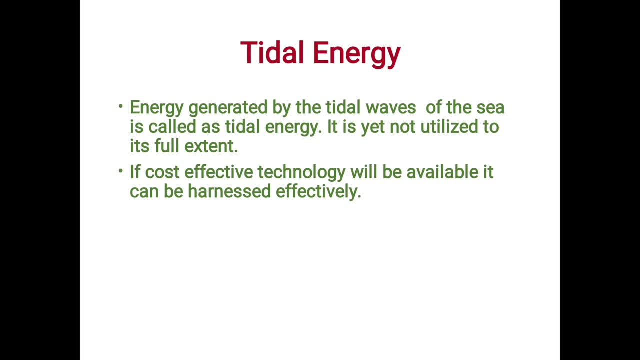 BSC 3, Semester 6.. Name of the paper: Environmental Geology. Name of the topic: Resource Management. Out of that we are going to learn energy resources. BSC 3, Semester 6.. Name of the paper: Environmental Geology. Name of the topic: Resource Management. Out of that we are going to learn energy resources.